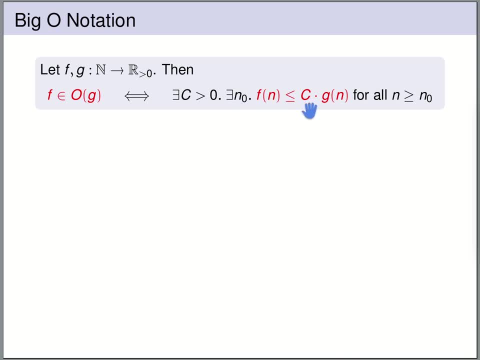 onwards, So starting from n0. this red condition holds for every n greater or equal n0.. So from n0 onwards, For g times, c is an upper bound for f. So what is this c here? This c means that in the big O notation we ignore constant factors. So f is in big O of g, if there exists some. 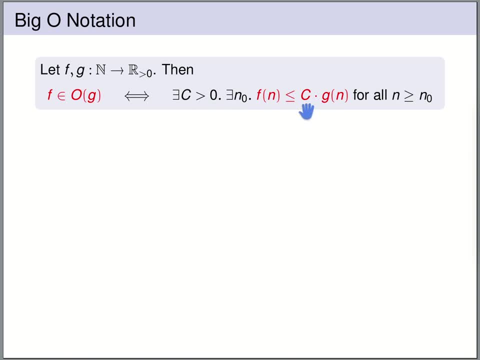 constant c, such that g times c is an upper bound for f from n0 onwards. Now why do we want to ignore upper bounds? because if you're looking at how many steps a Turing machine needs, then we don't want to count so extremely precisely whether there's one step more, one step less. 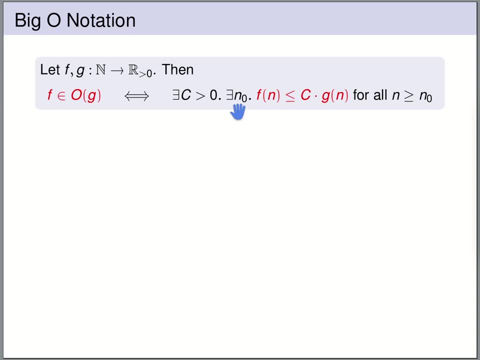 we want to give estimations, we want to say that the Turing machine needs a quadratic number of steps or cubic number of steps or exponentially many steps, but we don't want to be so extremely precise that we say that if the input is of a certain form, then it needs n square plus three. 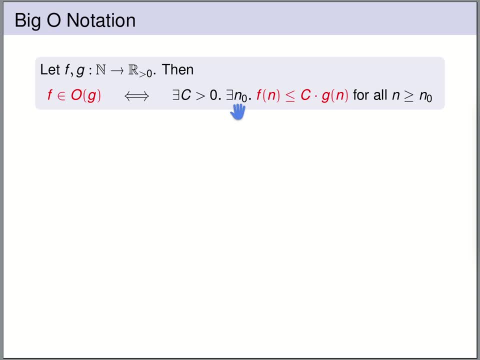 and so on. so we want to use this to give estimations upper bounds on the asymptotic behavior of our function f. so for instance n to the power a is always in big o of n to the power b, as long as b is as least as big as a. so as long as a is less equal than b. 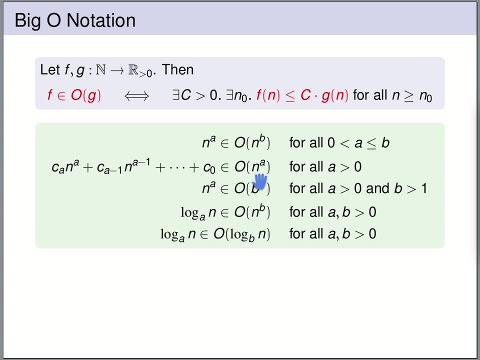 also the big o notation allows us to simplify polynomials. if we have any polynomial, so it does not matter what coefficients we have. with the largest exponent being a, then this polynomial is n to the a. thanks to these constant factors here we can ignore all the coefficients and we can ignore 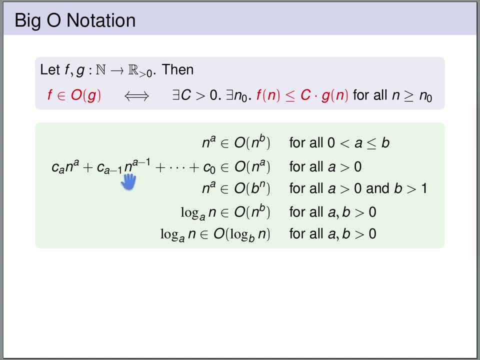 the smaller factors. so we can ignore the n to the a minus 1, n to the a minus 2 and so on. the only thing that matters for the asymptotic growth is the largest coefficient. but we can drop in n to the to the a, so the only thing that matters is n to the a. 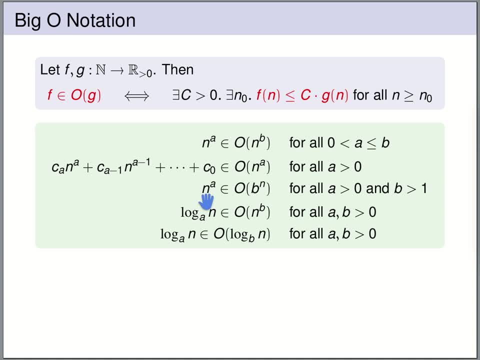 if we have a polynomial, then this polynomial always grows slower than an exponential function. so any polynomial will be in big o of b to the n as long as b is greater than one. so b to the n with b greater than one will grow exponentially. and that all when we give a exponential function that bigger. 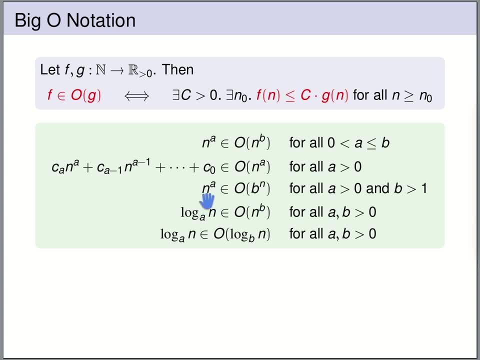 always grows asymptotically faster than any polynomial. Any polynomial, on the other hand, as long as b is greater than 0, will grow faster than a logarithmic function. So any logarithmic function log a of n will be in big O of n to the b as long as b is. 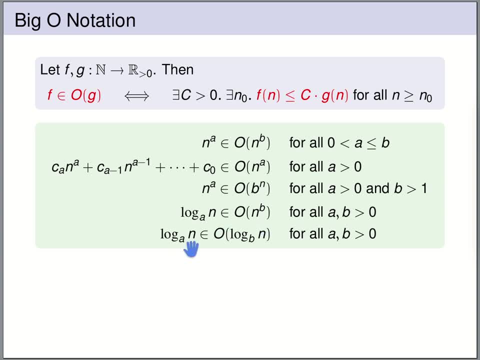 greater than 0. And for logarithmic functions the base of the logarithm doesn't matter, So we can freely exchange the base. as long as a and b are greater than 0, we have that log a. n is in big O of log b? n for arbitrary positive numbers a and b. 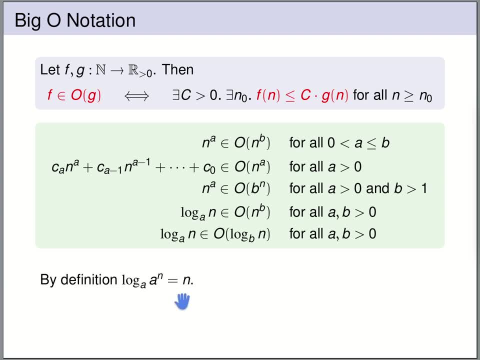 Let's prove this fact about logarithmic functions By the definition of logarithm. we have that the logarithm with space a of a to the power n is just n. So we also have that a to the power log a n is n. 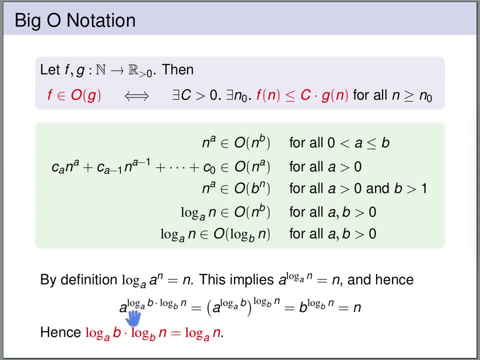 So we can compute the following: if we take a to the power, log a b times log b n, So if we have in the exponent a multiplication, then this is the same as taking twice exponentiation. So we can take a to the, So this is the same as a to the power. 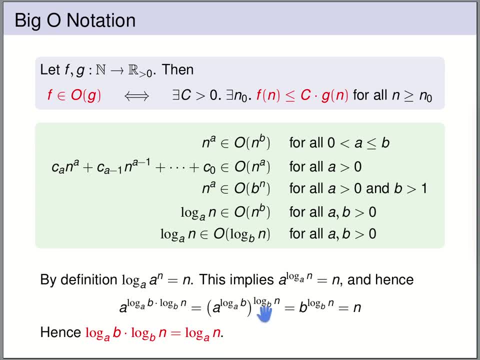 So this is the same as a to the power log a, b times log b n. a to the power log a, b is, as we've just said, this is just b. So we have b to the power log b n, b to the power log b. n, for the same reason, is just n. 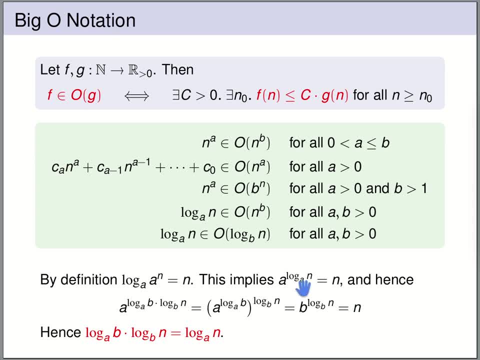 So this gives us n. So we have that. if you look at this, we get n. And if you look at this, we also get n. So we have that log a b times. log b? n is the same as log a? n. 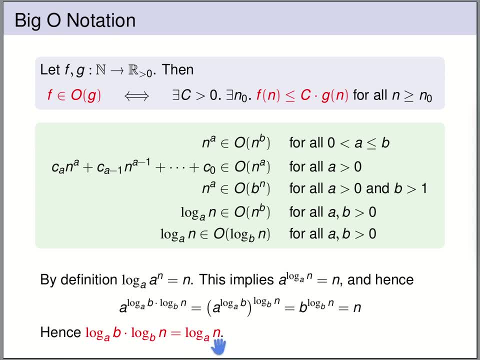 So this shows that the difference between log a n and log b n is just a constant factor, namely the factor log a b. So this log a b does not depend on n. So this is a constant. And since our big O notation has been obtained, we're also gonna notice that the зар é wird. 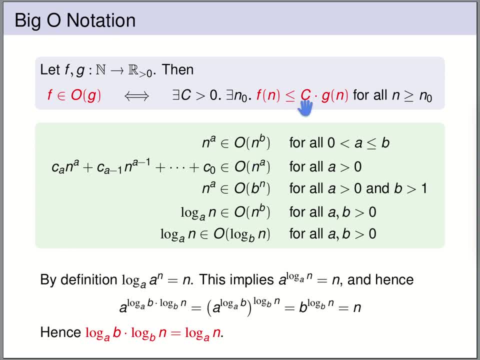 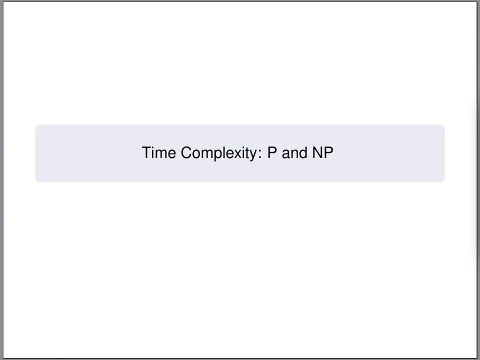 ignores constant factors. this is our c. here we have that log a- n is in big O of log b, n for any positive number a and b. First we are going to look at time complexity. So how much time is required to solve a certain problem? 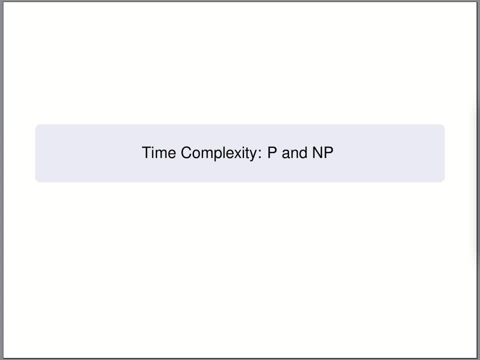 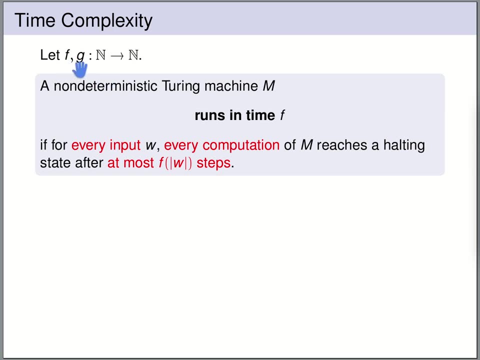 And in particular we are going to look at the complexity classes p and np. Here f and g are now functions over the natural numbers. We say that a non-deterministic Turing machine, m, runs in time f if for every input word w, every computation of f. 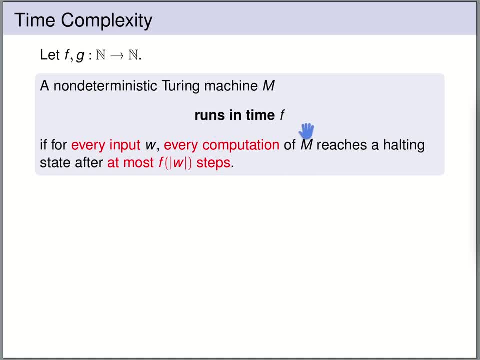 and here it is important to emphasize every computation, because we are speaking about a non-deterministic Turing machine. So for a given input word w, there can be multiple possible branching computations because of the non-deterministic choices in each step. So we require that every computation of m reaches a halting state after at most f of. 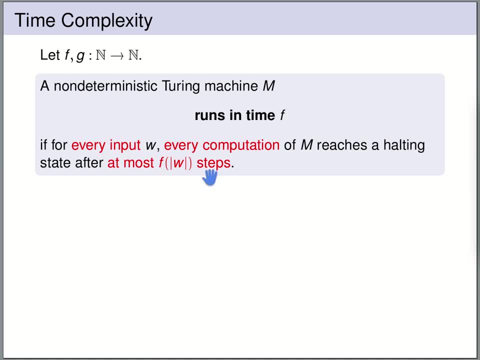 the length of m runs. So the number of steps may depend on the length of the input word. So, in other words, the function f gives us an upper bound on the number of computation steps in terms of the length of the input word, And this upper bound has to hold for every branch of the non-deterministic computation. 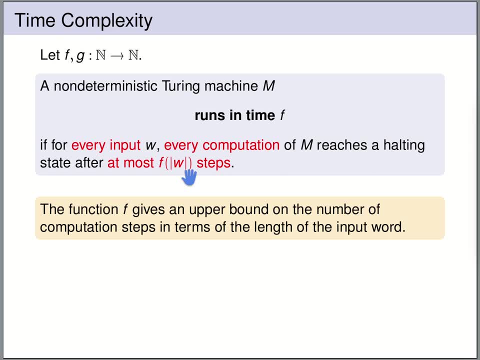 So not only for excepting computations but also for possibly non-excepting computations. No matter how we compute, we always have to stop after at most f of the length of w steps. We say that the Turing machine m has time. complexity O if the Turing machine runs. 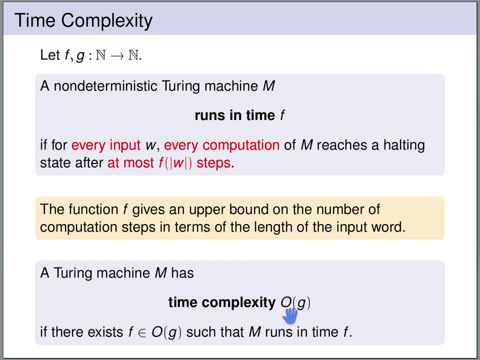 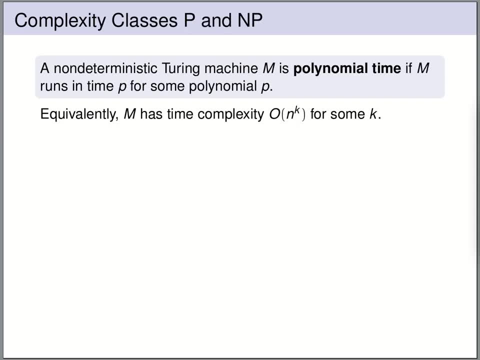 in time f for some f. in the set g We say that a non-deterministic Turing machine, m, is polynomial time. if there exists a polynomial p, such that m runs in time p, Equivalently we can say that the machine m has time complexity O for some natural number. 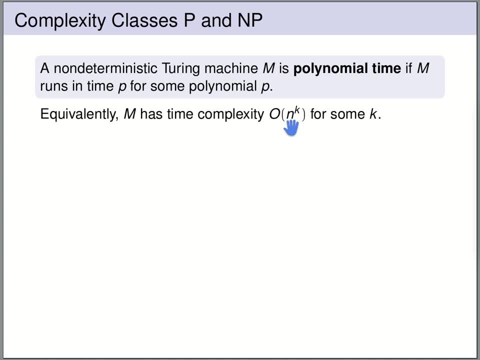 of steps. So a machine runs in polynomial time if there is a polynomial that gives an upper bound on the number of steps in dependence of the length of the input word. The class np is the class of all languages that are accepted by non-deterministic polynomial. 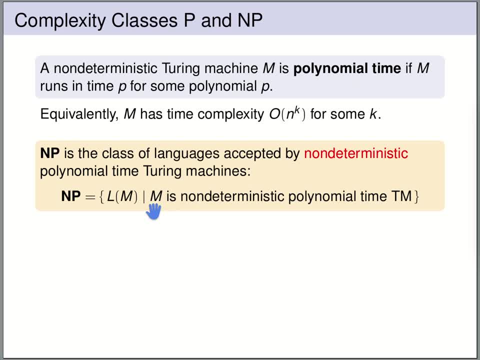 time Turing machines, And likewise We define p as the class of all languages that are accepted by deterministic polynomial time Turing machines. So both of these classes contain languages accepted by polynomial time Turing machines, And p allows non-deterministic polynomial time machines, whereas p only allows deterministic. 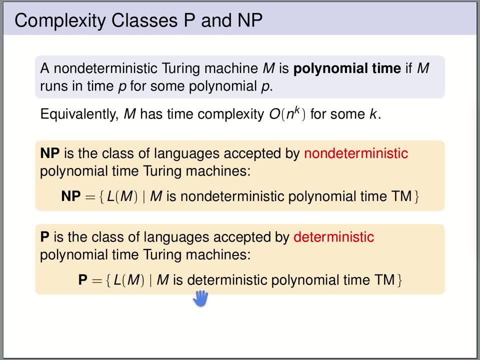 polynomial time machines. So since each deterministic Turing machine is antibodies to that normal daily steps, Each deterministic Turing machine is also a non-deterministic one. it follows immediately that p is a subset of np, But it is open up to today whether the classes p and np are actually the same. 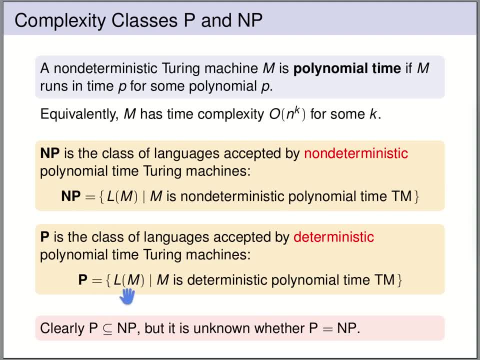 So whether every language in np is also in p. So what does this question mean? It means: can we translate: deixa de ovPD ba a-'s an affirmingdeml askba a sweet question, meaning that if m is a model PO in a given range from: 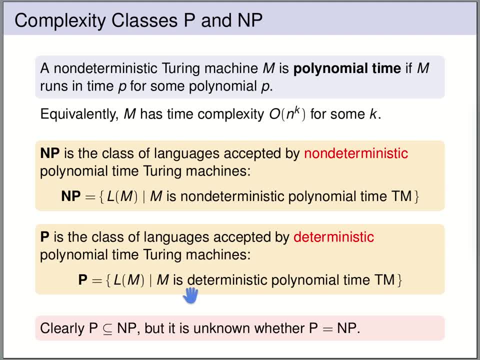 polynomial time Turing machine into a deterministic polynomial time Turing machine that accepts the same language. Up to today, it's not known whether this is possible. We have discussed that every non-deterministic Turing machine can be simulated by a deterministic one, But this simulation that we have discussed uses a breadth-first search, which requires 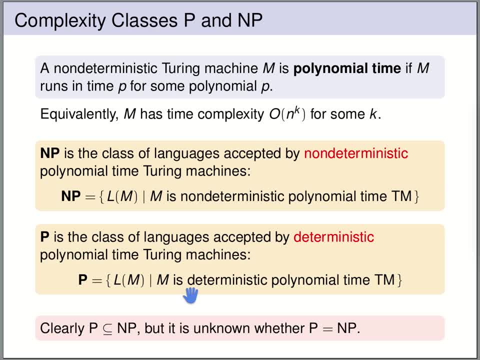 an exponential overhead for this simulation, So this ruins the polynomial time complexity. So the question is: can we do better? Can we do this simulation while keeping the polynomial time? A bit of time overhead is okay, but not an exponential one. The polynomial time overhead is fine. 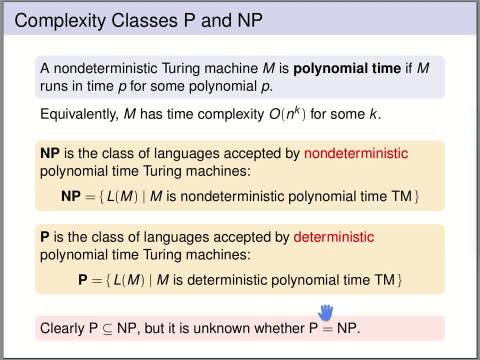 So up to today, this question is open And this question really has an explanation. It has an extreme practical relevance because encryption, basically, can be easily broken using non-deterministic polynomial time Turing machines. A non-deterministic machine can simply guess the encryption key. 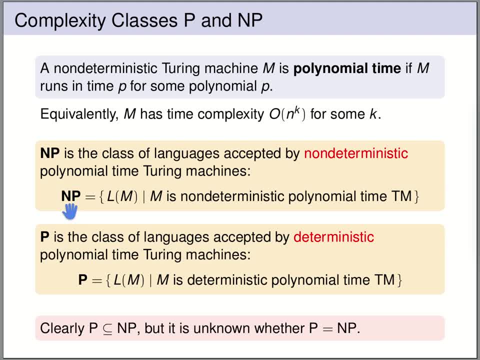 If you have an encrypted message. you don't have the key, but you would like to know what the original text was. If you would have a non-deterministic machine, then this non-deterministic machine could simply guess the password And decrypt the message. 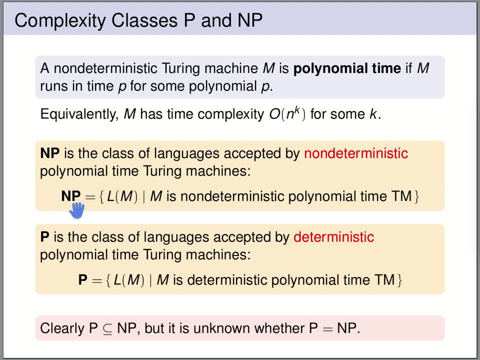 Now, non-deterministic polynomial time machines don't really exist in practice, But they are a nice theoretic concept. Deterministic polynomial time machines, they exist in practice. So if every non-deterministic polynomial time machine could be translated in a deterministic 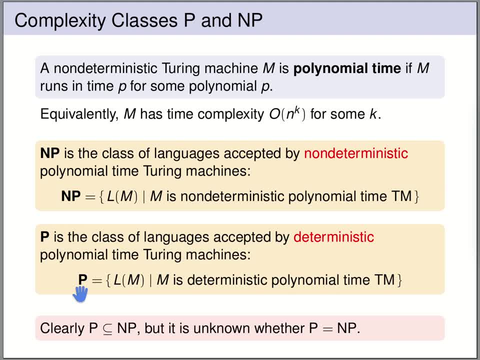 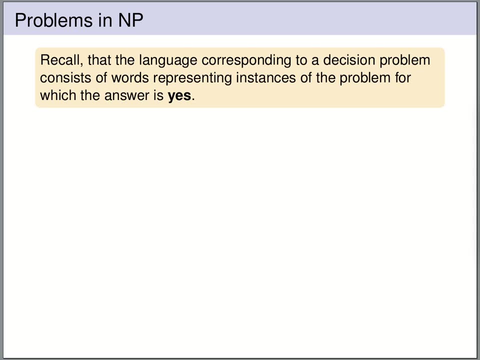 one, then it would mean that also deterministic Turing machines could break encryption in polynomial time, And that would really be dangerous. Let's have a look at some example: languages in the class NP. Recall that a decision problem is just a language. The words in the language describe instances of the problem for which the answer is yes. 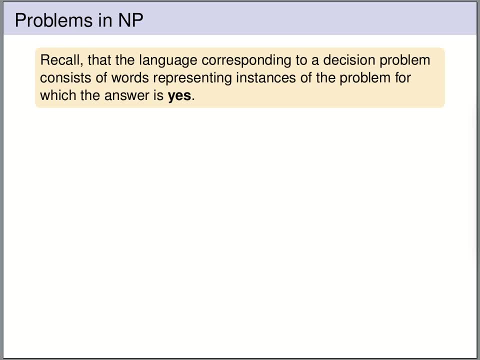 The words that are not in the language are those instances for which the answer is no, Intuitively a decision problem is in the class NP if every instance has a finite set of solutions and if correctness of a solution can be checked in polynomial time. 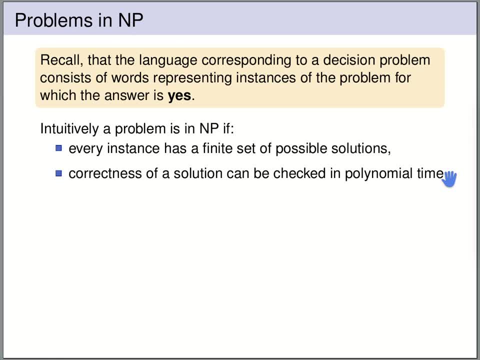 The class NP is defined by polynomial time non-deterministic Turing machines. We can use the non-determinism in order to guess a solution, And if we then can check in polynomial time whether this guessed solution is correct, then we are in the class NP. 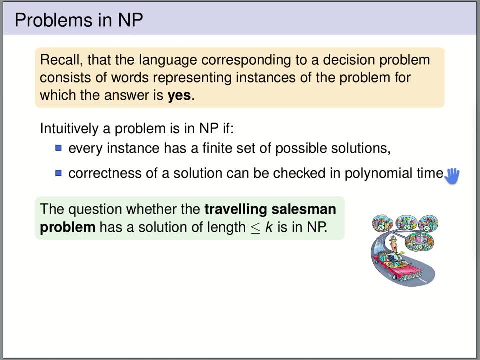 So for instance, this holds for the traveling salesman problem- We can check using a non-deterministic polynomial time Turing machine whether there exists a solution, a path of length at most k. The non-deterministic Turing machine can say that a non-deterministic Turing machine has. 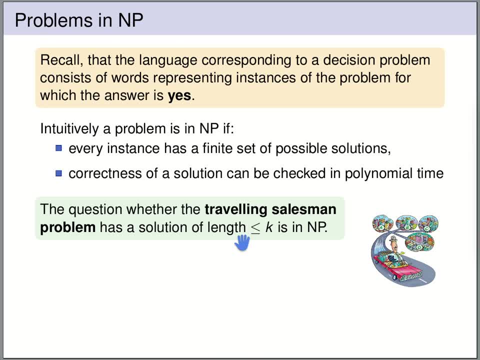 a path of length at most k. The non-deterministic Turing machine can say that a non-deterministic Turing machine has a path of length at most k. We can simply guess a path up to length k and then check whether this is a solution. 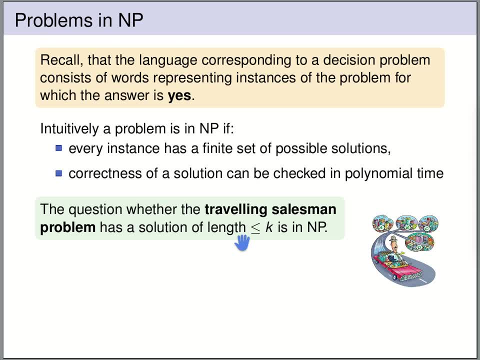 to the problem in polynomial time. Also, satisfiability in propositional logic is in the class NP. We can simply guess an assignment of the variables with true or false, and then we just need polynomial time to check whether the solution that we have guessed is correct. 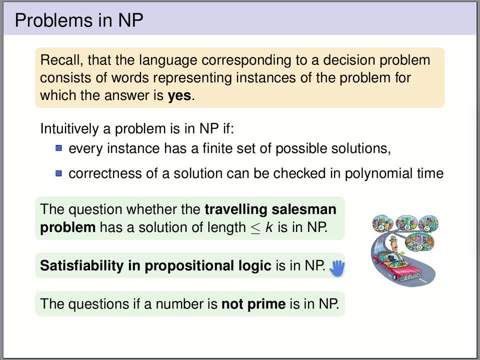 Also checking whether a number is not prime is in the class NP. Given a natural number, we can simply guess two factors and we can check whether the number is the product of these two factors in polynomial time. So also checking whether a number is not prime is in the class NP. 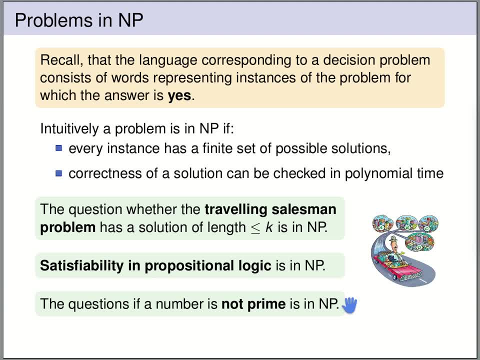 Actually, this problem has turned out to be not only in NP, But it has been shown in 2002 that this problem is in P. So there is a deterministic polynomial time Turing machine that decides whether a natural number is a prime number. 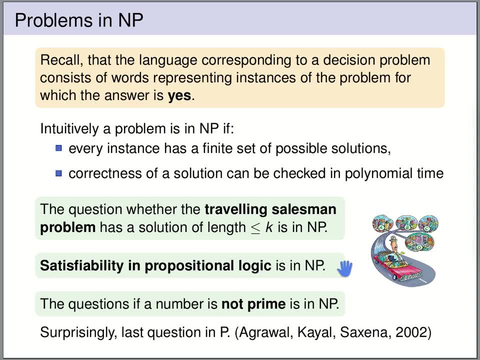 For the other two problems- the satisfiability in propositional logic and the travelling salesman problem- such solutions have not been found, So it's not known. It's not known whether they are in P. For these two problems the impact would be much bigger than for the prime problem. 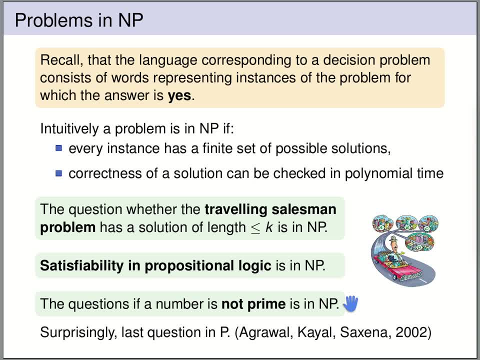 The prime problem was not known to be complete for the class NP. So we will see that the satisfiability in propositional logic and the travelling salesman problem are so-called NP-complete problems. If for these two problems the polynomial deterministic time solution would be found, 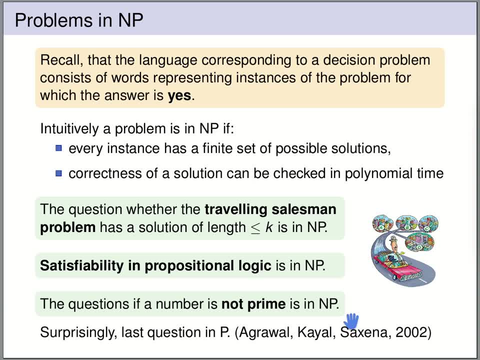 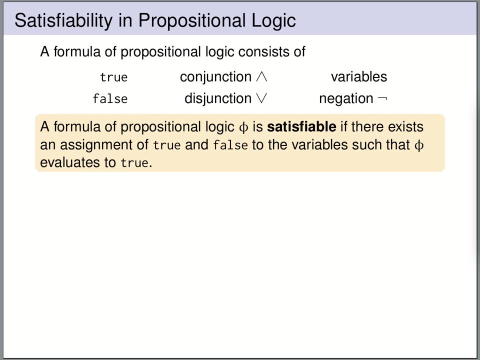 then it would mean that all problems in the class NP can be solved by a polynomial time deterministic Turing machine. We will later revisit propositional logic in this lecture, So let's quickly recall what it is about. A formula in propositional logic is built from the following building blocks: 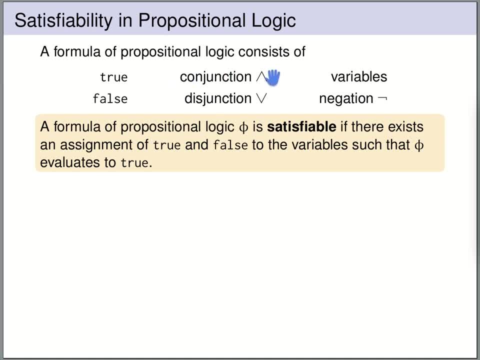 We have constants, true or false. We have conjunctions and disjunctions that are binary operations. Think of conjunctions as AND and disjunctions as OR. We have propositional variables and we have negation. A formula in propositional logic is called satisfiable if we can assign true and false. 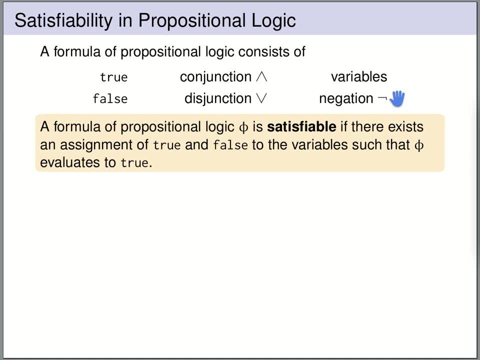 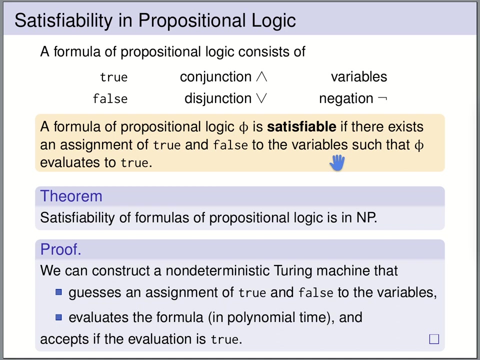 to each of the variables in such a way that the formula evaluates to true. The question whether a formula is satisfiable is NP, So it's in the class NP And the proof is what we've just sketched on the last slide. 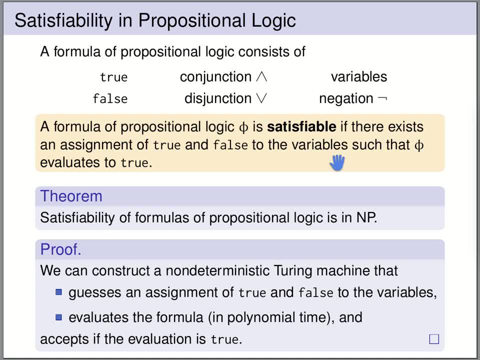 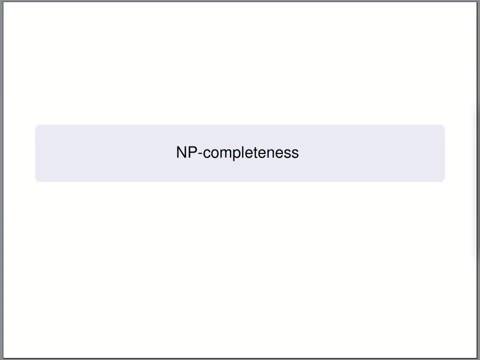 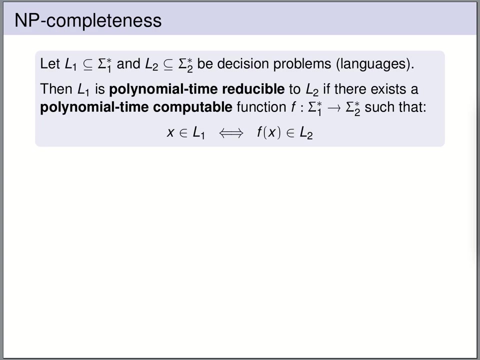 Namely, we can construct a non-deterministic Turing machine that guesses some assignment of true and false to the variables and then evaluates the formula in polynomial time, And if it evaluates to true then it accepts the formula. Next we are going to look at certain problems in the class NP that are called NP-complete. 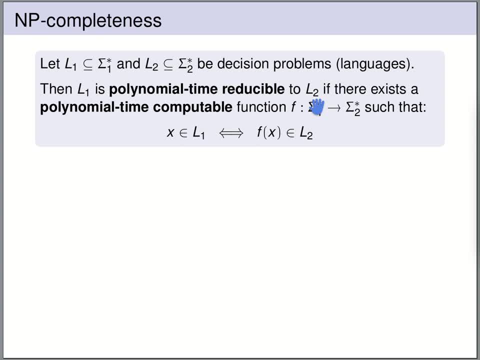 Let L1 and L2 be decision problems. So L1 is a decision problem over the alphabet sigma 1. And L2 is a decision problem over the alphabet sigma 2.. L1 is said to be polynomial time reducible to L2 if there exists a function from words. 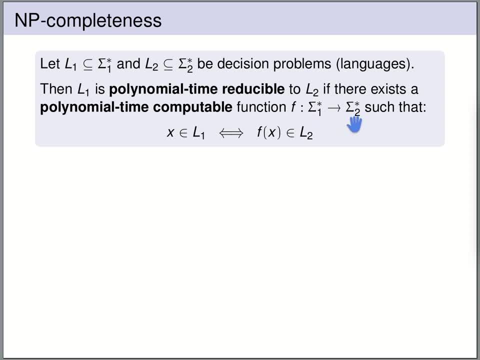 over the alphabet sigma 1 to words over the alphabet sigma 2, such that this function f is polynomial time computable. So there is a deterministic Turing machine that computes f in polynomial time, And for every word x there is a function f. 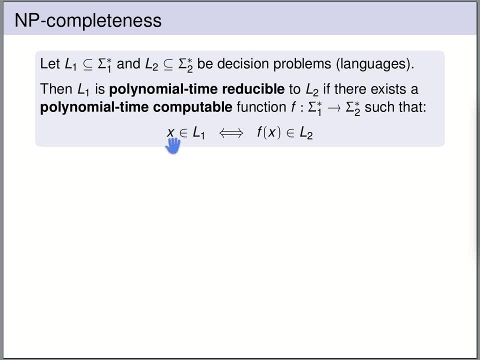 For every word x over the alphabet sigma 1, we have that x is a member of L1 if, and only if, f is in L2.. So intuitively, this means that if we want to decide whether x is in L1, we can simply: 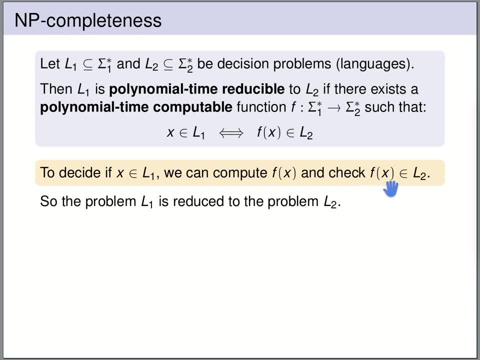 compute f and check whether f is in L2.. So we have reduced the question about membership in L1 to a question about membership in L2.. We therefore say that we have reduced the problem L1 to the problem L2.. We have a polynomial time reduction from L1 to L2.. 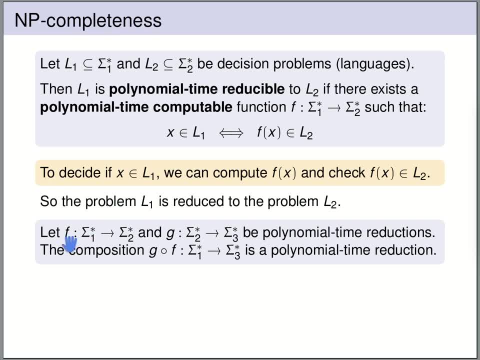 If we have two polynomial time reductions, a polynomial time reduction f from alphabet sigma 1 to sigma 2, and g from sigma 2 to sigma 3, then the composition of f and g is a polynomial time reduction from the alphabet sigma 1 to the alphabet sigma 3.. 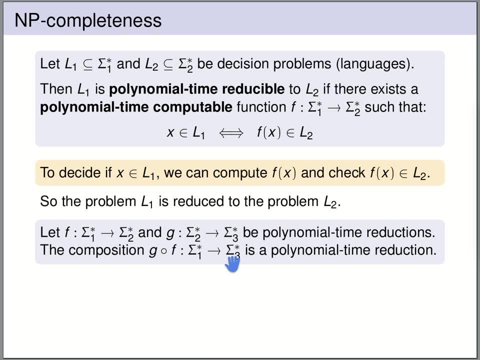 The underlying reason here is that if we have two polynomials, then the composition is again a polynomial. A language L in the class NP is said to be NP-complete if every language in NP is polynomial time reducible. So if we have an NP-complete language, then every problem in NP can be reduced to this. 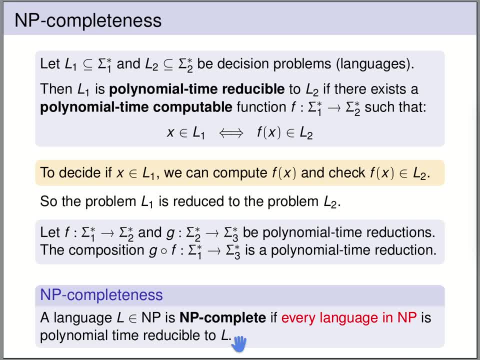 NP-complete problem in polynomial time. These NP-complete problems and the polynomial time reductions really have also a strong practical relevance. If you have some NP-complete problem, then the polynomial time reduction can be reduced to some NP-complete problem and you find a very efficient way of solving it. then it 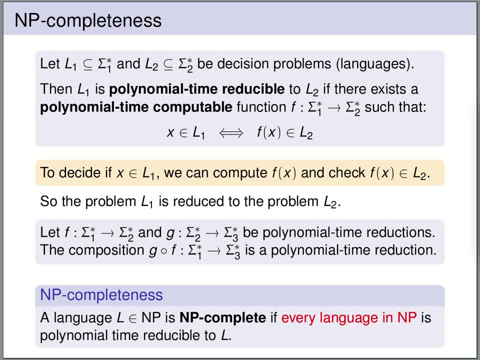 means that also the other problems in the class NP can be solved efficiently by translating it into your particular NP-complete problem. In particular, if we would be able to find a deterministic polynomial time algorithm that solves some NP-complete problem, it would mean that suddenly all the problems in the 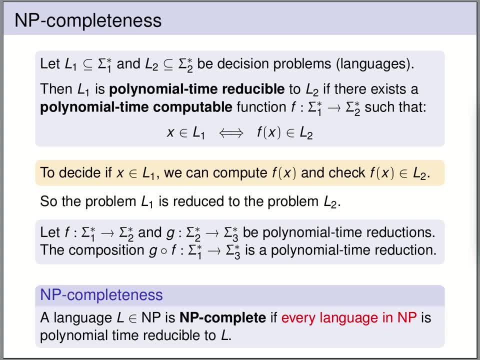 class NP are solvable in deterministic polynomial time, So P would be equal to NP. As mentioned before, this is still open, so such algorithm has not been found yet and probably it doesn't exist. However, from the practical perspective, there have been practically efficient algorithms. 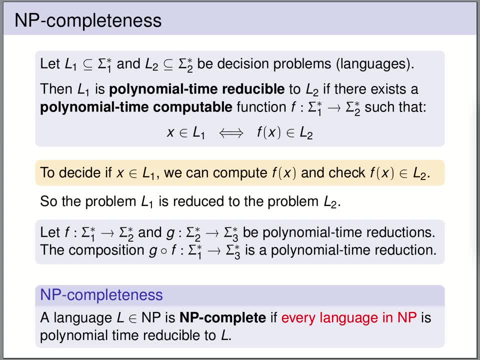 found for some NP-complete problems, in particular for the satisfiability of NP-complete problems. There are programs out there called SAT-solvers that are very efficient in determining whether a formula is satisfiable and, if so, computing a satisfying assignment. Since satisfiability of propositional logic is an NP-complete problem, it means that we 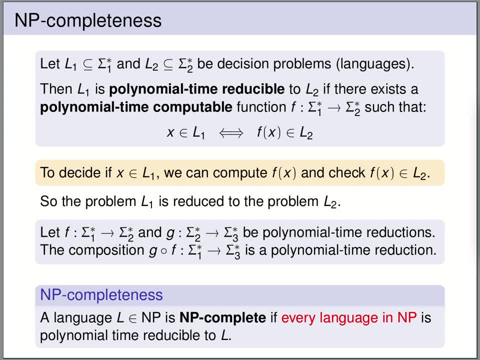 can solve other problems in the class NP by translating them into NP-complete problems, And then we can ask these SAT-solvers whether there is a satisfying assignment for this formula, and if so, we can translate it back to a solution of our original problem. 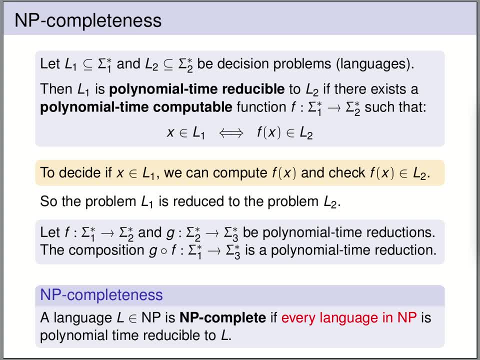 And this is actually a very efficient strategy that is applied numerous times in industry at the moment. So, for instance, for deciding how to lay out certain components on a chip. for example, Intel, AMD and others use SAT-solvers to solve these kinds of problems. 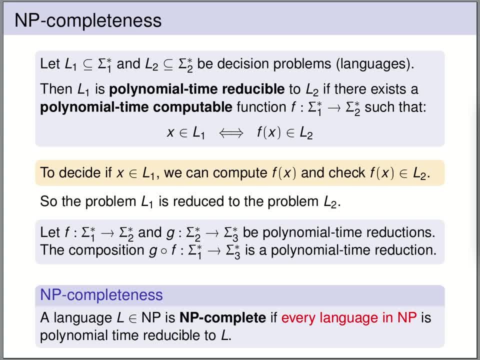 And also in other areas, SAT-solvers have turned out to be more efficient than dedicated solutions that have been developed in many areas. So there are various NP-complete problems where dedicated solutions have been developed over decades. In the last decade SAT-solvers have come along and now suddenly the most naive translation 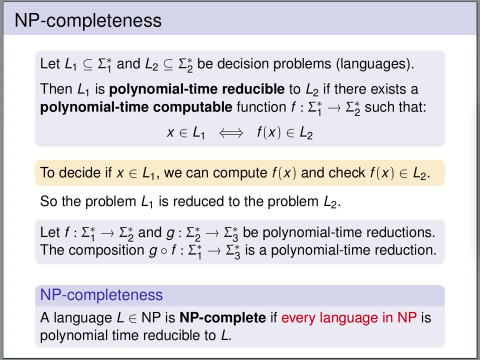 of these problems into propositional logic and, using a SAT-solver, outperforms all of the solutions that have been developed in these dedicated areas over the decades. So if you are working on a NP-complete problem and you think about writing your own solver, 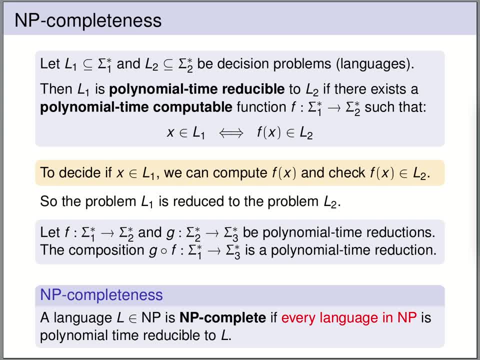 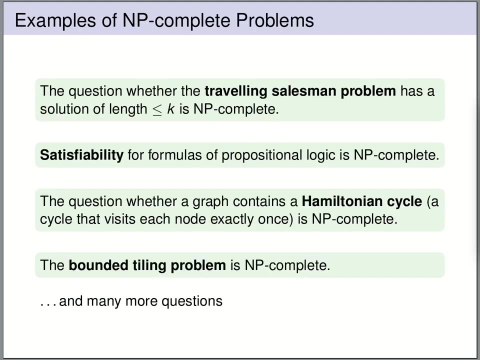 rather think about translating it into a satisfiability problem and try out SAT-solvers. Very likely the translation to SAT-solvers will outperform any dedicated solution that you can come up with. So there are various different problems that have turned out all to be NP-complete. 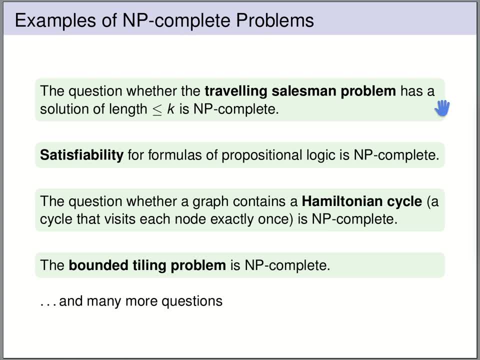 We've already mentioned the traveling salesman problem, the satisfiability of propositional logic. There are many other problems that have turned out all to be NP-complete. There are many other problems that have turned out all to be NP-complete. Also, the question whether a graph contains a Hamiltonian cycle. 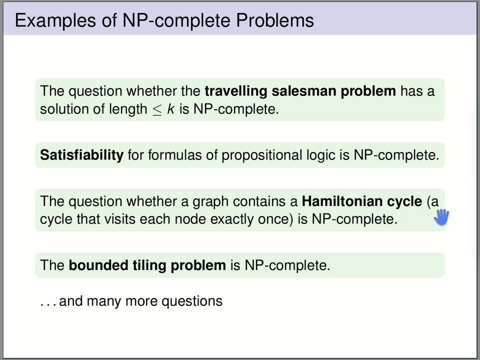 So a Hamiltonian cycle is a path through the graph that visits each node precisely once. This question is also NP-complete, And in this lecture we will still see the bounded tiling problem, a kind of puzzle, that is also NP-complete. 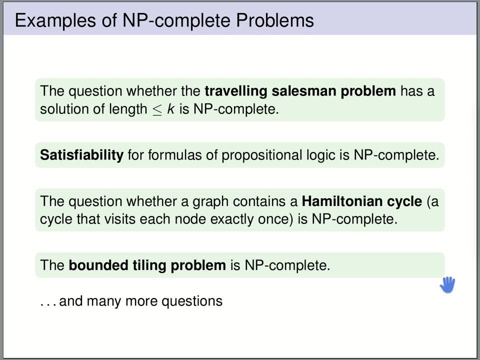 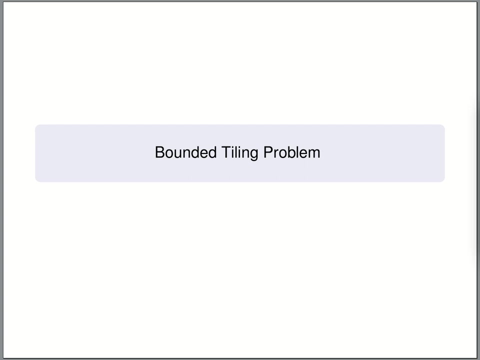 And, like these problems, many more questions are NP-complete. Usually any kind of combinatorial questions turn out to be in this class NP, and often they turn out to be NP-complete. So let's have a closer look at one of these NP-complete problems, namely the bounded tiling. 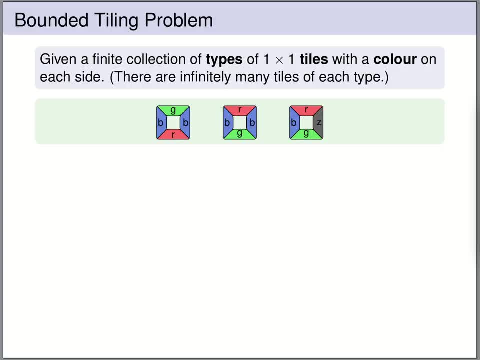 problem. The bounded tiling problem is a puzzle. The tiles that we use in this puzzle are these square tiles. They have colors on each of the sides, and we will also write a word on each side to emphasize what color it is. Now, the main idea of the bounded tiling problem is that we use these tiles and we try to 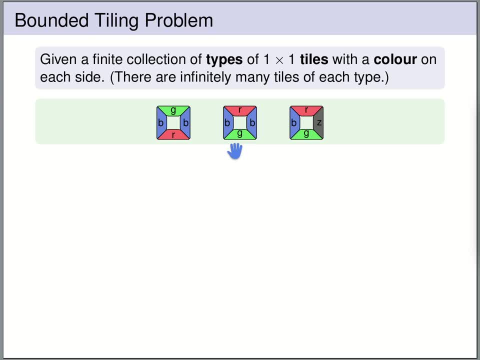 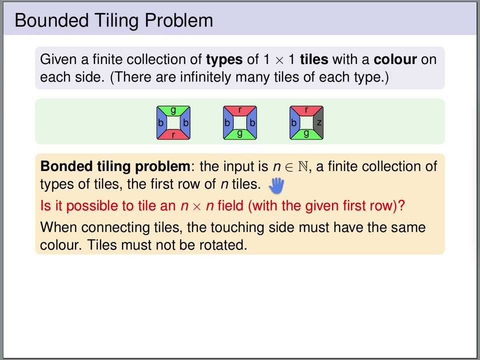 fill some area with it, And when two tiles are next to each other they are called bounded tiles. When two tiles are next to each other, then the touching sides must have the same color. So, to be more precise, the input for the bounded tiling problem in the instance consists: 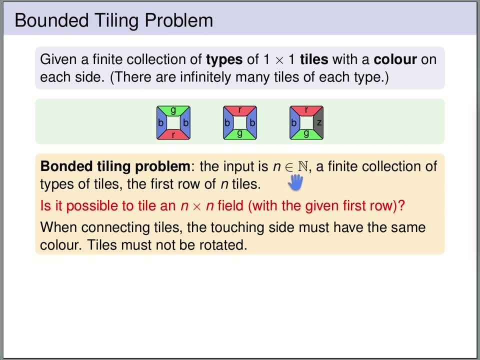 of a natural number, n, a finite collection of such tile types, and we can use each of these tile types arbitrarily often. So we assume that we have an infinite number of copies of each tile type and we are given the first row of n tiles. 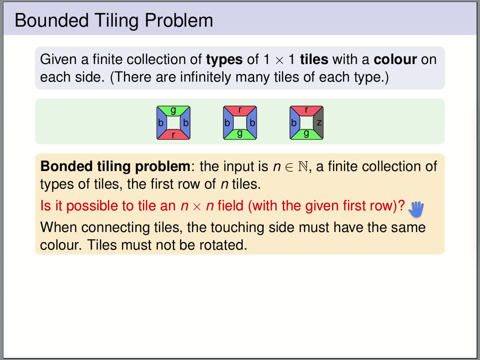 So the first row is given and the question is: can we tile an n times n field with the given first row and only using the given tile types When two tiles are next to each other- the connecting sides, the touching sides must. 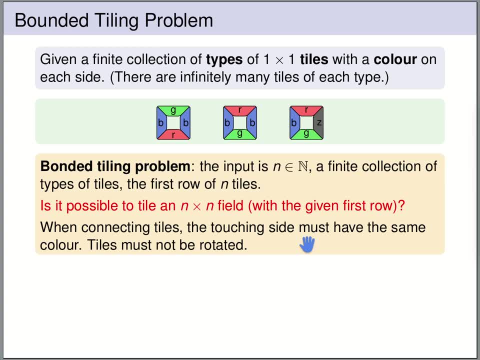 have the same color and we assume that the tiles are not allowed to be rotated. This is simply for simplicity. You can also make a variant of this puzzle that is NP-complete, in which you can rotate the tiles, But for simplicity, we assume that we are not rotating here. 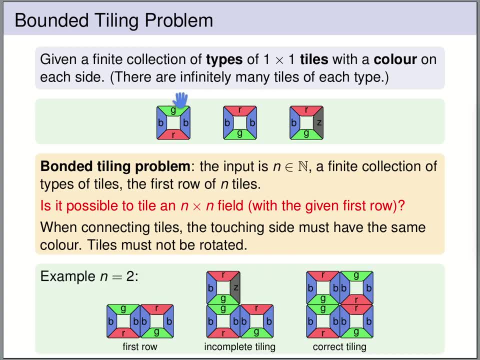 So, for instance, we assume that we are not rotating. So, for instance, we assume that we are not rotating. So, for instance, we assume that we are not rotating. So, for instance, if we are given these tile types and we are given this first row, so 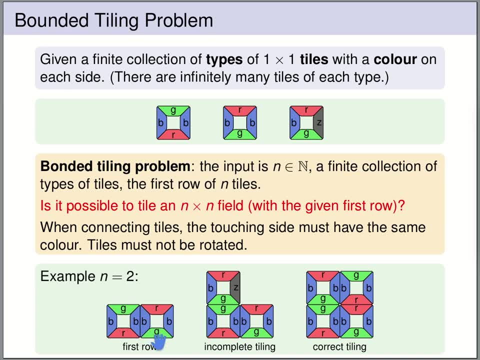 now n is two and this is our first row. so the question is: can we fill a two times two field with this first row? One thing we could do: we have two tiles that have green on the bottom, so we have a choice. 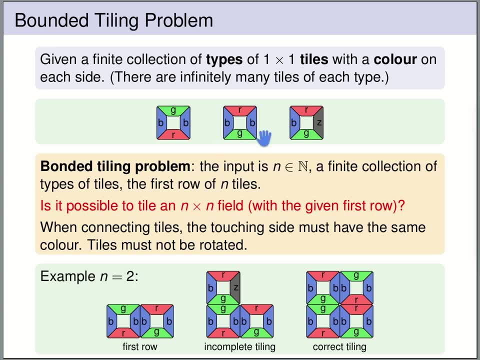 between two tiles to put on top here. We can either use this or this. If we use the right hand, we can either use this or this. If we use the right most one, then we get this situation and now we have a black side on. 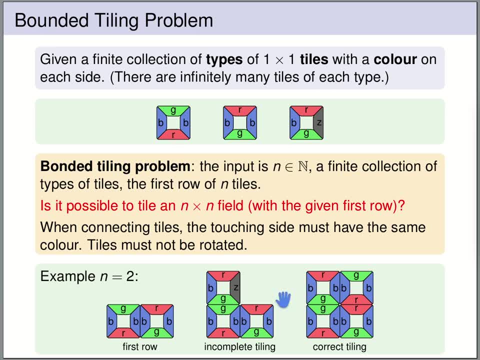 the right and there is no tile that we could put in this upper corner. So this attempt cannot be completed. It is an incomplete tiling, but we can tile differently. We can put: on the upper left we can put this tile, and on the upper right we can put this. 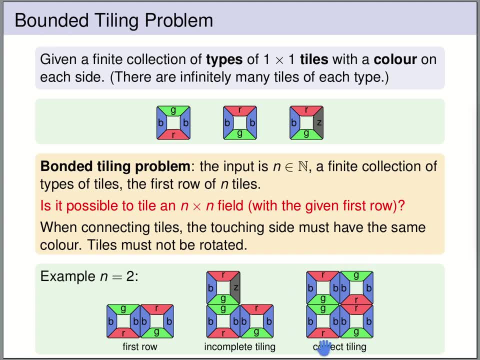 tile and now we have blue tiles on both sides, ples, And now we have a complete tiling. We have completely tiled a 2x2 field with the given first row and all the touching sides have the same color: Here green, here blue, here red and here also blue. but that was already given. 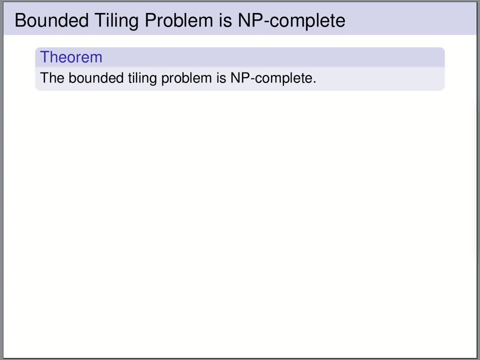 So now we want to prove that the bounded tiling problem is indeed NP-complete. So there's two parts which we have to show. First we have to show that the bounded tiling problem is in the class NP And we have to show that every problem in NP can be reduced to the bounded tiling problem. 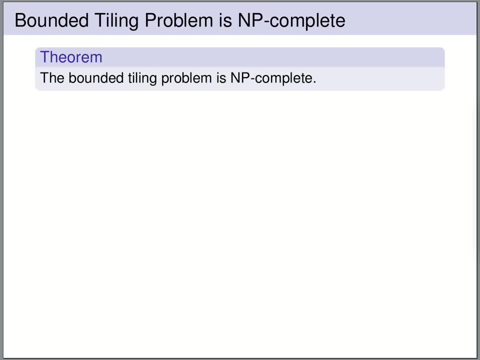 in polynomial time. Let's start with the first part of the proof. We show that the bounded tiling problem is in NP, So we have to show that a non-domestic polynomial time Turing machine can solve the bounded tiling problem, And the idea is simple. 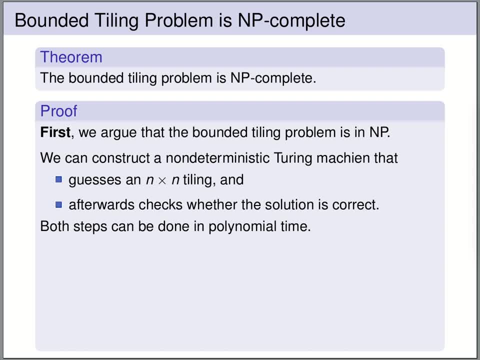 We construct a non-domestic machine that in the first step guesses a tiling, guesses an n times n tiling. So it walks over the field and it assigns tiles to each place And afterwards the non-domestic Turing machine changes. It checks whether the guessed tiling is indeed the correct solution. 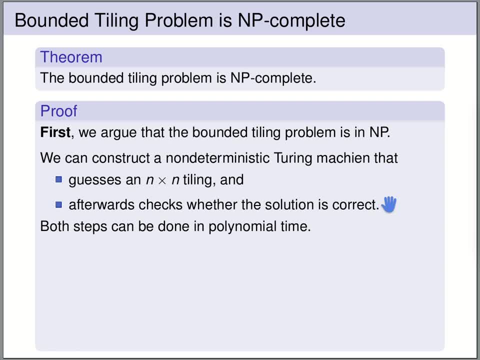 So it checks whether all the tile types that are next to each other match, so that the colors on the touching sides are the same, And the second step can indeed be done in polynomial time. Therefore, we have a polynomial time Turing machine that can solve the bounded tiling. 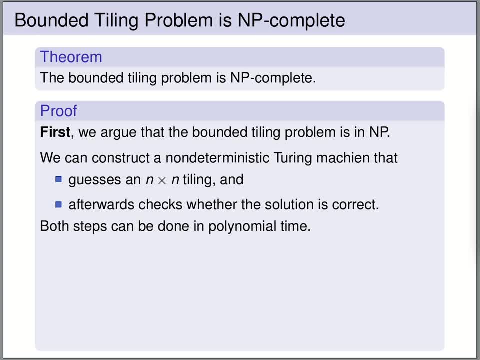 problem. Thank you. Next, we have to show that the bounded tiling problem is indeed NP complete. So we have to show that every problem in the class NP can be reduced to the bounded tiling problem in polynomial time. Every problem in the class NP can be accepted by a non-domestic polynomial time Turing machine. 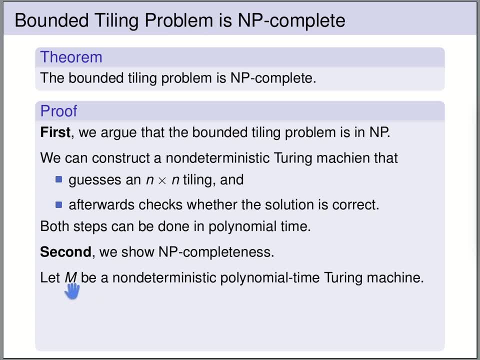 So we take a non-domestic polynomial time, Turing machine m. Since this is polynomial time, it runs in time p for some polynomial p, And we now show that the question of membership in the language of this Turing machine can be reduced to the bounded tiling problem in polynomial time. 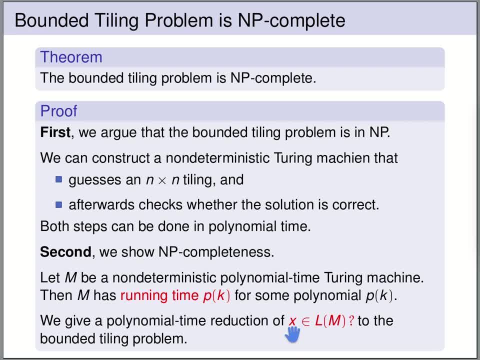 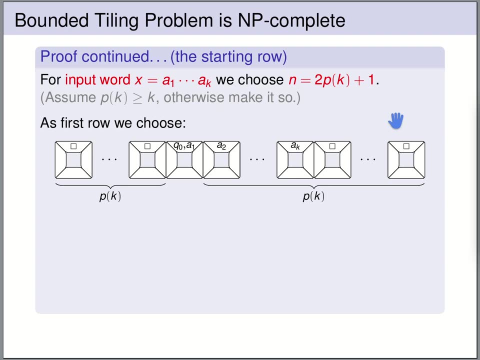 So for a given word x, we will reduce the question whether x is in the language of the Turing machine To an instance of the bounded tiling problem. So let's assume that our input word x consists of letters a1 up to ak. 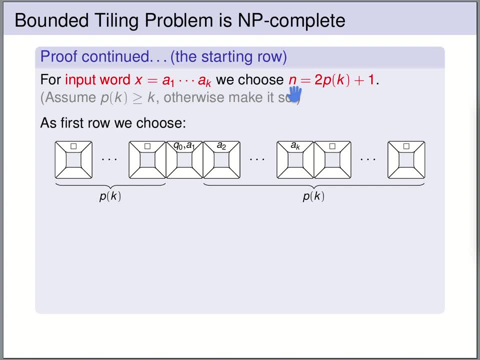 And for our size of the bounded tiling problem n, we choose two times p of k plus one. So k is the length of the input word, P is the running time of our Turing machine. so P is an upper bound on the number of steps that our Turing machine does. We take 2 times P because of the following: 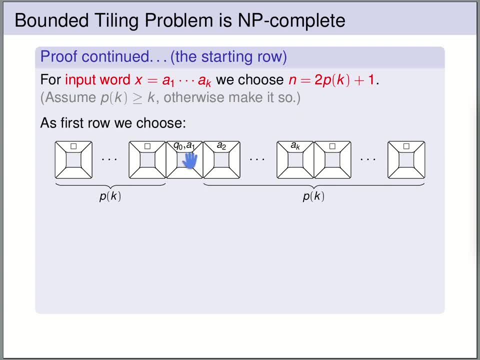 Our Turing machine starts on the first letter of the input word, on A1. But we don't know whether the Turing machine will move left or right, or maybe both. If the Turing machine indeed does, PK steps as the upper bound maximally allows and if the machine always. 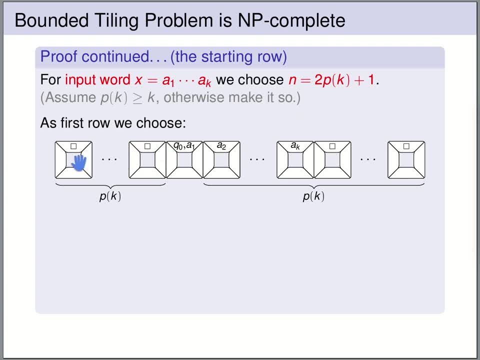 walks to the left, then we need PK blank symbols to the left. If the machine always walks to the right, then we need that we have PK symbols to the right available for the Turing machine to walk on. So we take our letter A1 and we make sure that there is PK. 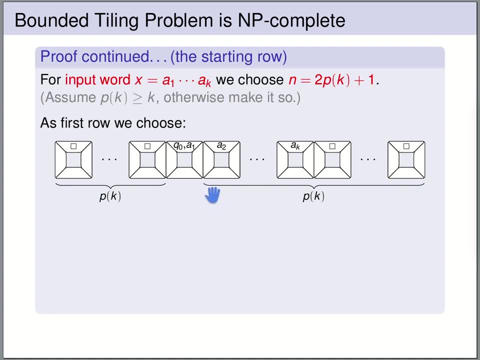 symbols to the left and PK symbols to the right, such that there is enough space for the Turing machine to walk until it stops in at most PK steps. So if you look at the length of this, then we have here one time PK, one time more PK. 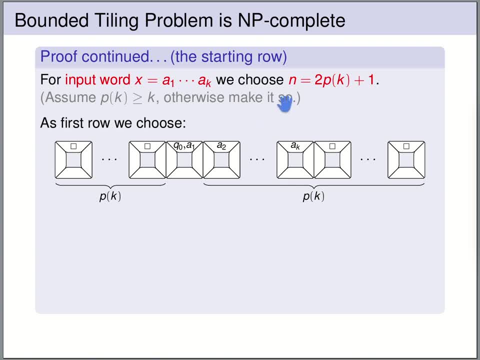 plus one letter, so 2 times PK plus 1.. This explains the size of our bounded tiling problem N. We choose as the first row of our bounding tiling problem this configuration. So we have PK blank symbols, Then we have tiles. that basically. 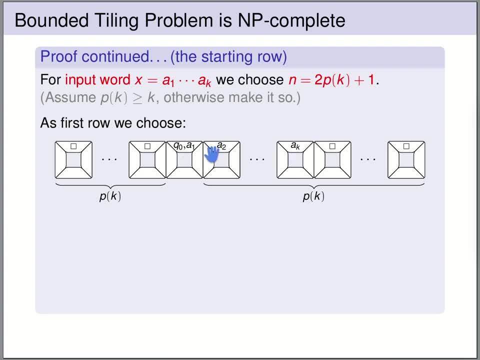 contain on the top our input word A1, A2, A3, up to a A Only on the first letter of the inputşaard. exciting competition as liquidity available. area 5,. we have also additionally Q0, written, Meaning that this is the place where currently the head of our Turing machine stands. 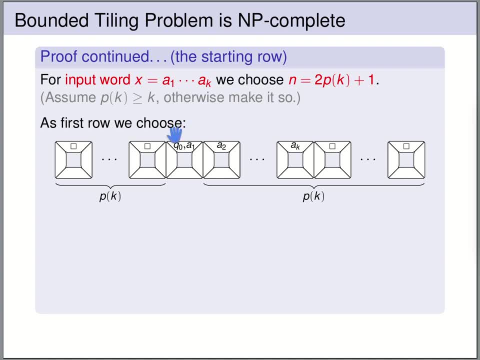 Assimilating inputs and ancients. We place A1,, A2, A3 is also present- on the top of the letter. we have such a state of the Turing machine And we fill up with a number of blank tiles, if needed, in order to make this at least the length pk. So what kind? 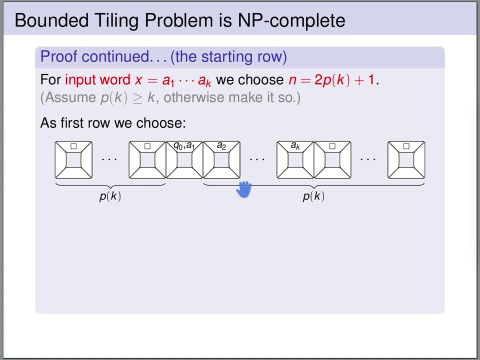 of tiles. do we need to construct this first row? We need tiles with a blank symbol on top as a color. we need tiles with color q0a for an input letter, and we need tiles that just have an a on top and nothing else. So these words that we 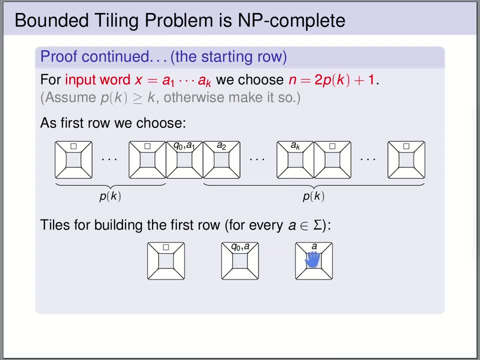 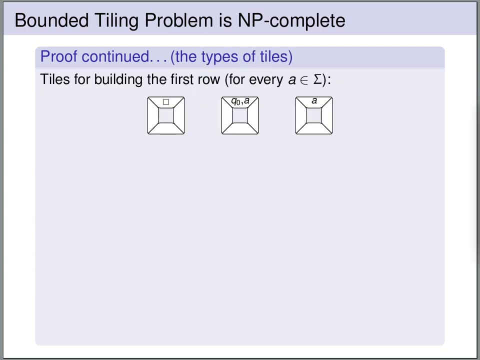 write here. these are the colors of the sides, And you can think of this just as having no color, or think of any color that you like. So we have these tiles of types for building our first row. We have these tiles for every a in our input alphabet sigma, Next to these tiles for the first. 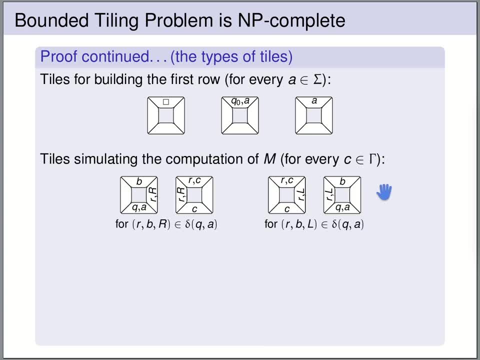 row. we also need tiles for simulating the computation of our Turing machine. These are these tiles. we have them for every transition of our Turing machine and for every c in our tape alphabet gamma. So if we have a transition of the following form, if we are in state Q, we read an A. 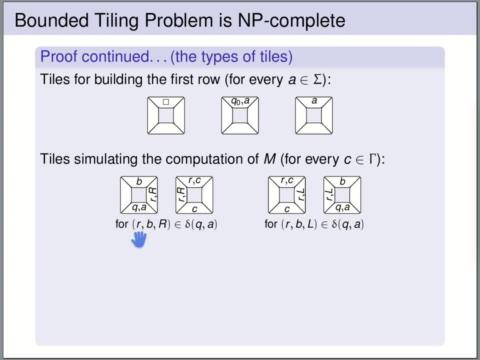 and we have a transition that switches from state Q to state R, overrides A by B and moves to the right. then we have these two tiles for every C in gamma. So we see here that on the bottom row our Turing machine is in state Q and we stand. 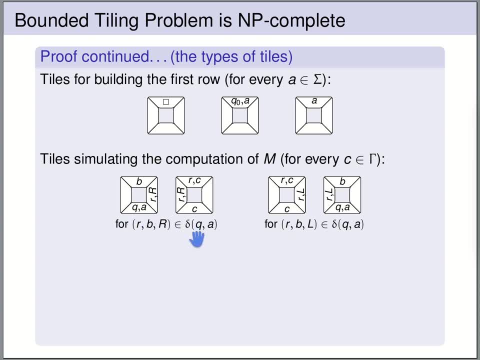 on a symbol A. So we have the case that we are in state Q and we read an A On the top, we see that the A has been overridden by B, and on the top row we also see that now the Turing machine is in state R and it has moved to the right. 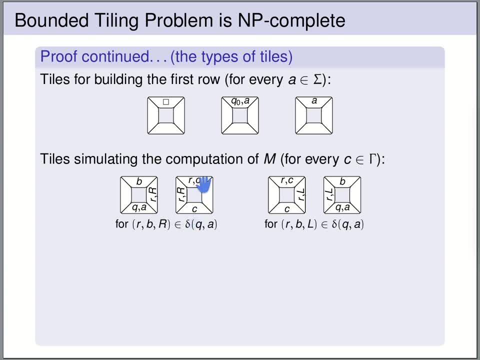 And this works. we have these tiles for every C in gamma. Okay, Now how do we make sure that we indeed have moved to the right? I've said we moved to the right, but these tiles, they are not really. it's not ensured. 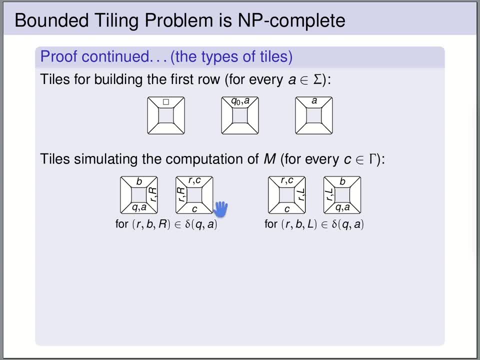 that we use them next to each other. However, this is ensured by the following annotation, namely, on this left tile, on the right-hand side, we write the color R for the state that we switched to and capital R for the direction of moving to the right. 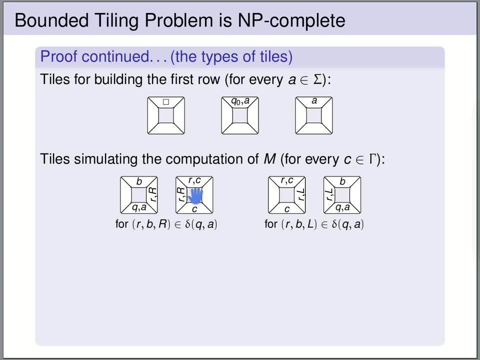 This has to be matched by the same color, namely by a tile of this form which has lowercase R and capital R written on the left side. So only if these two match we can put them next to each other. And seeing such a state R and the movement direction R on this tile means that we move. 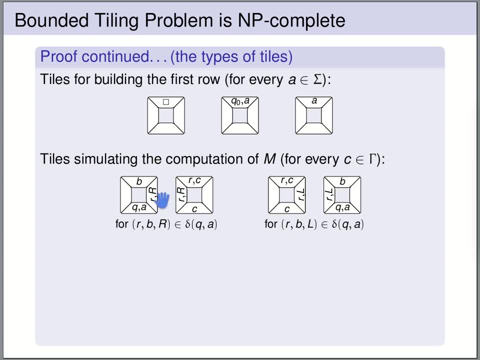 to the right and we switch to state R. So that means that on the top of the right we must have then the state R, And likewise we have this for moving to the left. If you're in state Q, we read the letter A and we have a transition that switches from. 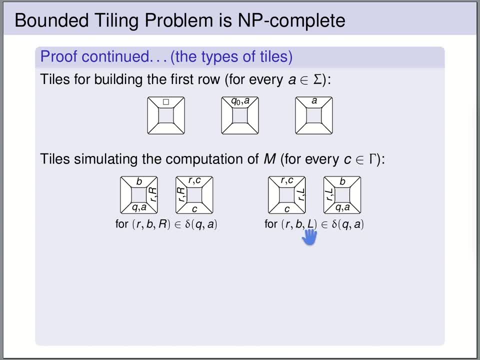 state Q to state R overrides A by B and we move to the left. Then we have again a tile where we are in state Q, read an A, We overwrite A by B And for any C from the tape alphabet we have a tile like this: 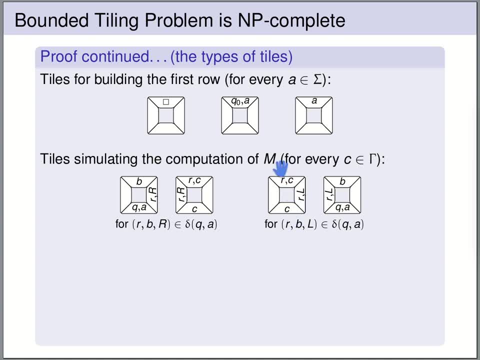 The C stays, but additionally we put R here. That's the state that we switched to. And again, how do we make sure that this tile is really used at the left side of this tile? It's by using these annotations. Here we have an annotation R, L. R is the state we switched to. 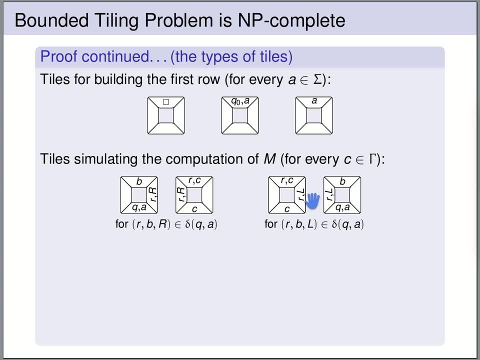 L is the direction. So if we have this on the right side, then it must be matched by another tile where the same annotation is on the left side. So these two tiles have to be used next to each other And having a state R and L annotation means that the left tile must have the state R on. 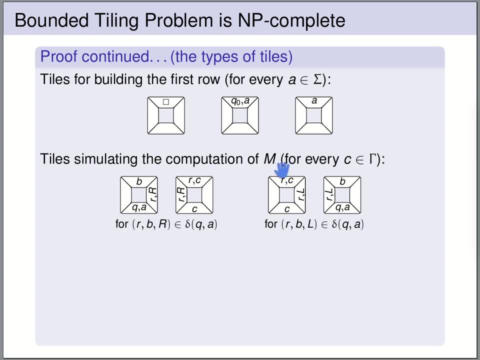 the top because we have moved to the left. Okay, So we have these tiles. for every transition, We have two tiles and for every letter C of the input alphabet, And then we need some additional tiles that allow us to leave the tape unchanged. 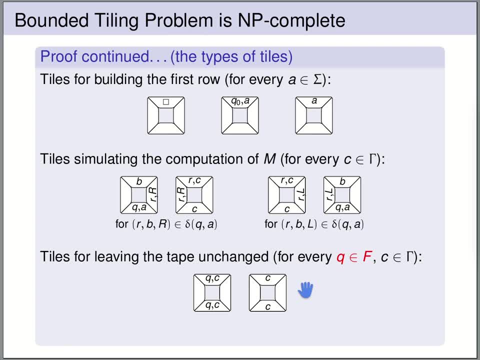 So that's where the Turing machine does not operate. So the tiles that are to the left or to the right, We have tiles of the form. Bottom we have color C and top we have color C, for every C in the tape alphabet. And for the tiles which have also state annotations of the Turing machine, we can copy this without. 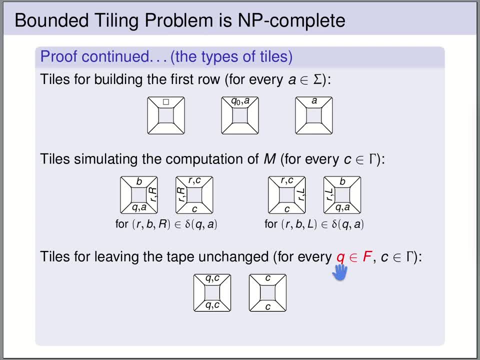 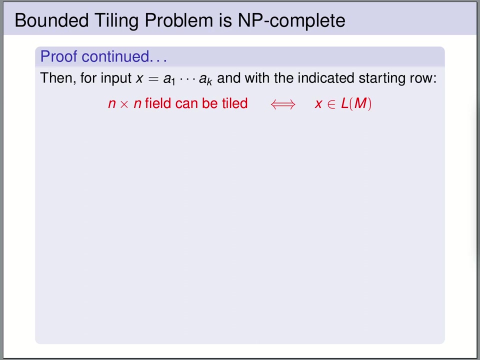 changing if we have a final state. So if Q is final, then for any tape alphabet letter C. we also have a tile that has at the bottom annotation QC And at the top also Okay, And also the color QC. For the bounded tiling problem that we have just created, it can be shown that an N times. 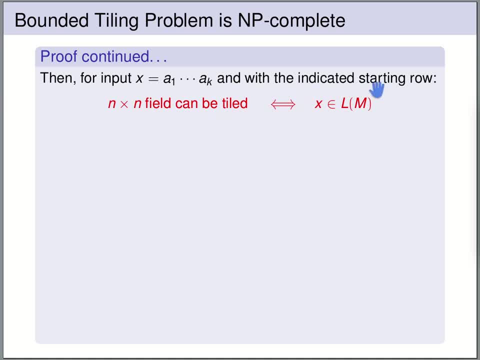 N field can be tiled with the given starting row if, and only if, the word X is in the language of the Turing machine. So we have reduced the question about membership in the language of the non-dynamistic Turing machine to solvability of the bounding tiling problem. 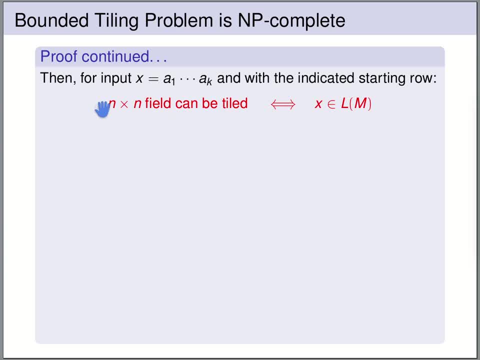 So why does this work? The idea is that such a tiling simulates a computation of our Turing machine on the input X. The input X we have encoded into the starting row and we've chosen the tiles of our bounded tiling problem in such a way that a good tiling 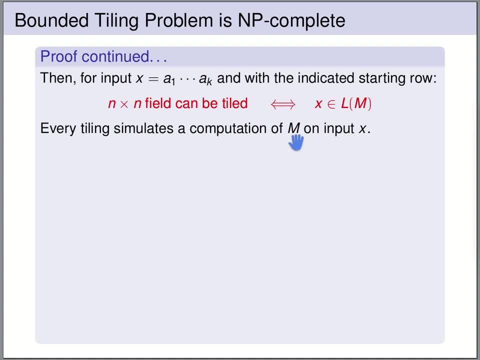 Simulates the computation of the Turing machine M, Since our Turing machine computes at most PK steps, But the size of our bounded tiling problem N is two times PK plus one, So there's more rows than computation steps of our Turing machine. This means that only the first PK tiles. 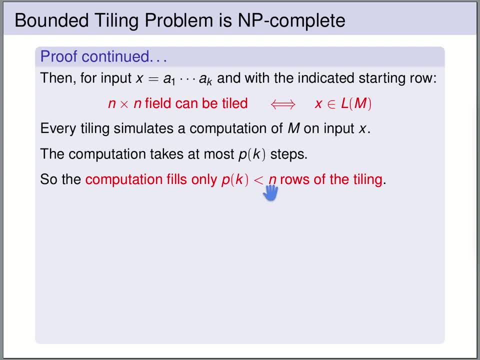 And this is smaller than the number of rows- will be filled by computation steps. So the only way to complete the tiling is by using these kind of tiles where the Q is a final state. So we can only complete the tiling if, and only if, the Turing machine reaches a final. 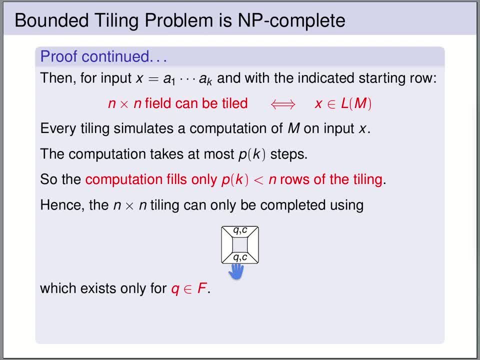 state, And that means that We have a solution to this, This bounded tiling problem, if, and only if, the word X, which is encoded in our starting row, is in the language of the machine. So, to summarize, we have translated the question of membership in the language of a non-termistic. 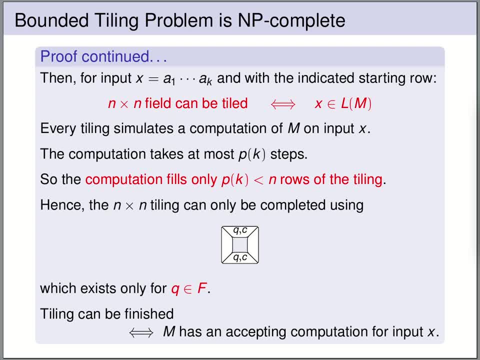 polynomial time Turing machine to instances of the bounded tiling problem And our reduction is indeed a polynomial reduction because the tiles that we use for our bounded tiling problem they only depend on the Turing machine, They do not depend on the input word. 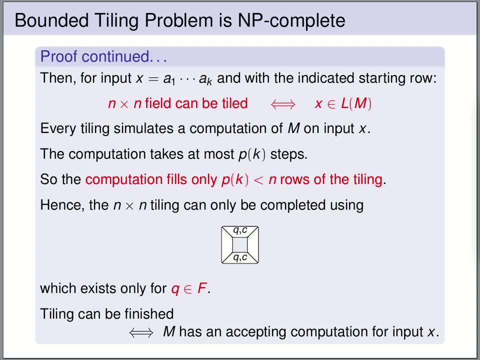 So the number of tiles that we have is constant. The size of the bounded tiling problem is polynomial in the length of the input word because we have chosen N to be two times PK. So that's the problem. Okay, So we have P of K plus one, and the P of K is the running time of our polynomial time. 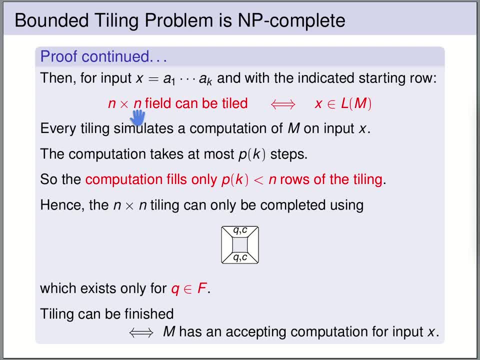 Turing machine. So the size N is a polynomial with respect to the length of the input word. So our starting row has polynomial size with respect to the length of the input word. So we have a polynomial translation from the membership question to instances of the bounded. 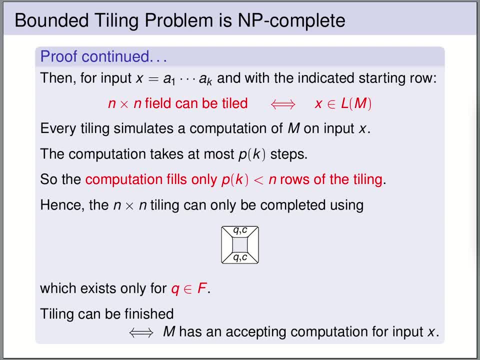 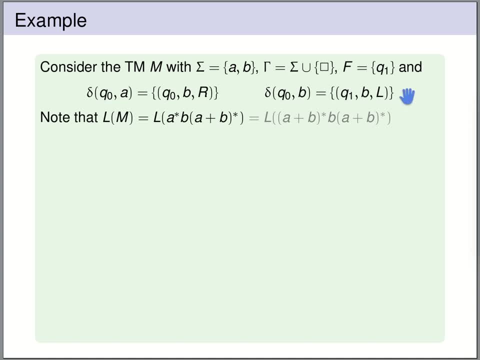 tiling problem. So, for example, consider this Turing machine. It has two states, Q0 and Q1.. It has the input alphabet A, B. The tape alphabet additionally contains the blank symbol And we have only one accepting state. one final state, Q1.. 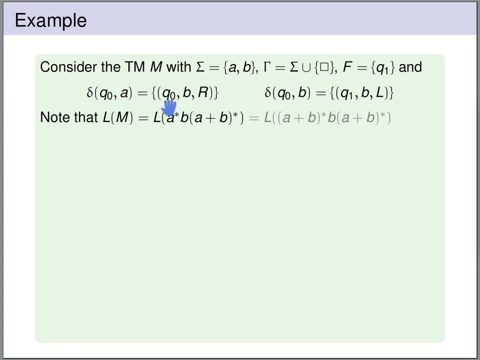 If we are in state Q0, we read an A, We stay in Q0.. We read an A, We stay in Q0.. We overwrite A by B and we move to the right. If we are in state Q0, we read the B, We switch to Q1. 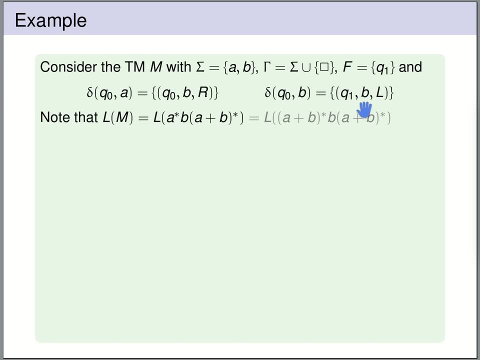 We overwrite B by B, So we leave it unchanged And we move to the left. So what is the language of this machine? It walks over the word until it finds a- B. If it finds a B, it switches to an accepting state. 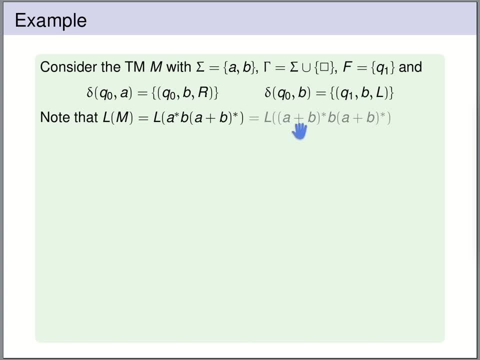 So the language accepted by this Turing machine consists of all words that are over the input alphabet A, B and that contain at least one B. So how many steps does our machine do at most? It does at most as many steps as the length of the input word. 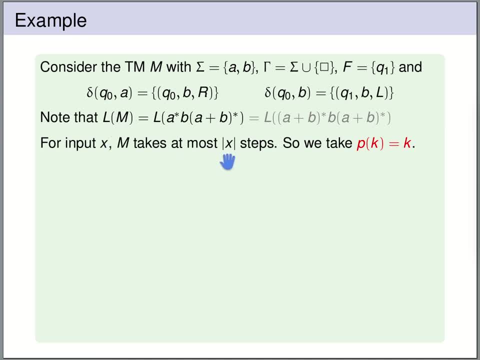 So if our input word is X, then our machine M does at most the length of X steps. So for the running time of the machine we can take, the polynomial defined by P of K is equal to K. So if we have an input word of length K, we do at most K steps of our Turing machine. 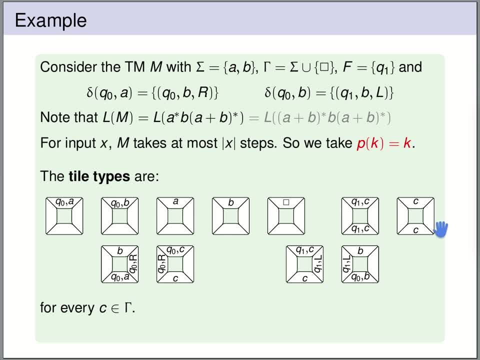 Now for the bounded tiling problem. we use the following tile types. These are the tile types for simulating this Turing machine. We have these first tiles here for defining our start starting row for encoding the input word X. We have tiles that have an A on the top because A is an input. 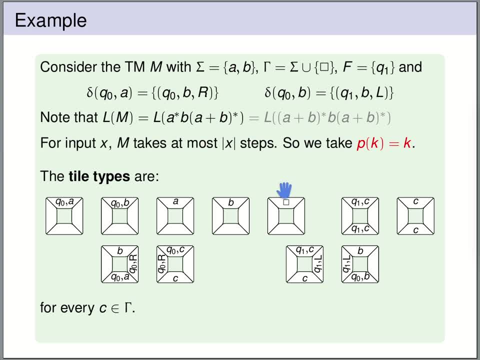 letter B on the top because B is an input letter. blank symbol on the top. We have tiles Q0A for the case that we want to start our Turing machine and state Q0 on the first letter of the word is A, And we have Q0B in case the first letter of our word is B. 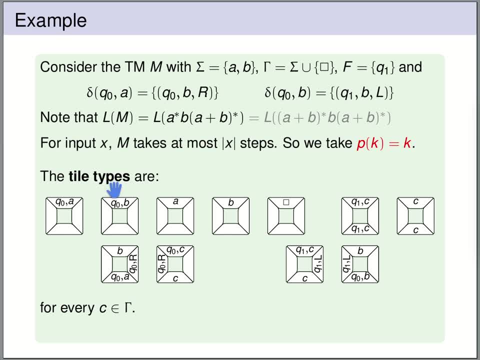 And we want to start the Turing machine in starting state Q0. Then we have these tiles for every C in the tape alphabet Gamma. These tiles here on the bottom are for simulating the computation of our Turing machine. So for the first transition we are in state Q0. 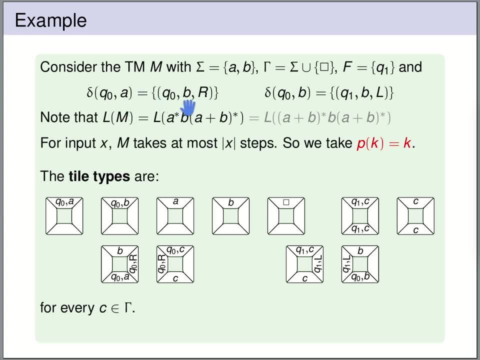 We read an A. We read an A, remain in state Q0,. we overwrite A by B and we move to the right. This corresponds to these tiles. We are in state Q0,. we read an A. The A is overwritten by B. We stay in state. 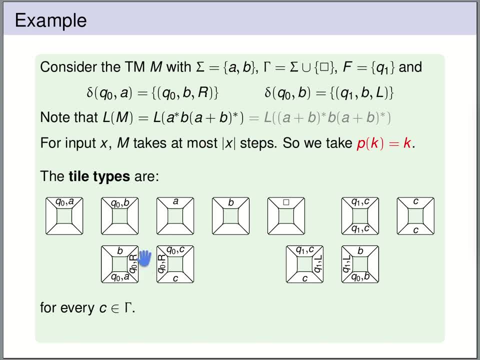 Q0 and we move to the right. That's indicated by the R. So then we have these matching tiles, We are switching to Q0, we move to the right. So we now have a Q0 here on the top And we 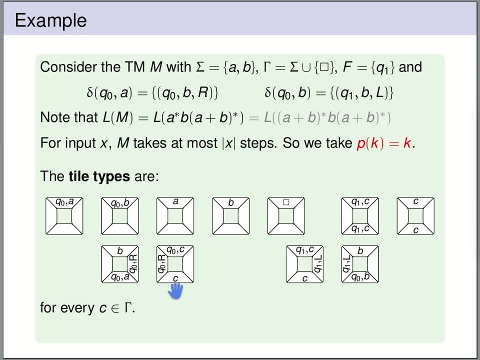 have this for any letter C in the tape alphabet. So no matter what letter C we had right of the head, we want to be able to move to the right. And similarly for the second transition. we are in state Q0,, we read a, B, we switch to Q1,, we leave the B and we move to the left. 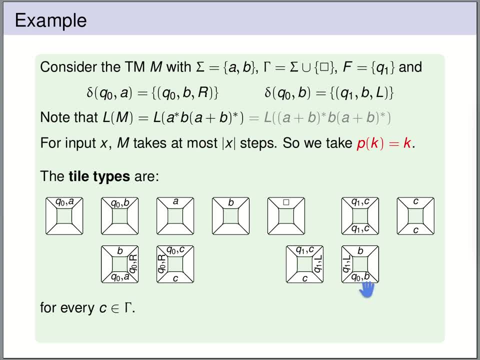 We have these tiles. We are in state Q0, we stand on a B, we leave the B, We switch to Q1 and we move to the left And matching, we have this side. We switch to Q0,, move to the left. So now there's a Q0 on top here And we have this for any letter C in our 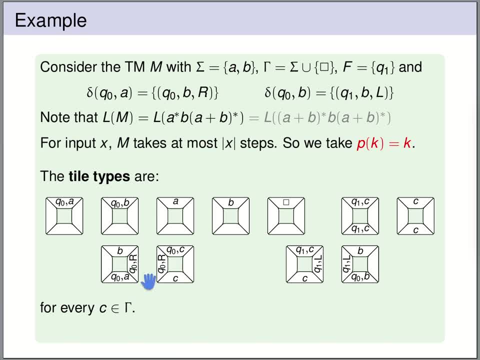 tape alphabet. So these tiles simulate a transition with respect to this transition. These tiles can simulate this transition. And then we need some tiles for copying the tape where there's no computation happening. So that's these tiles. They can just copy an arbitrary letter C of the tape alphabet from. 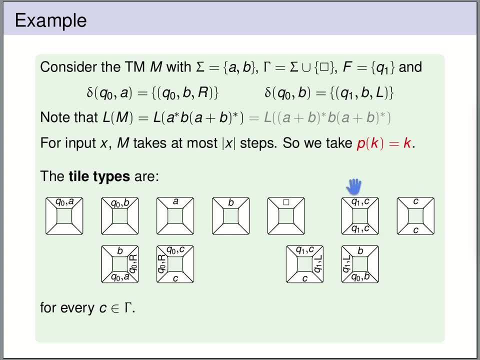 the bottom configuration to the top configuration And we have these tiles. That's, if our computation was successful- has ended in the final state. We have only one final state here. It's Q1.. So whenever we have Q1, for any letter C, we have this, And we have this, And we have this And we. 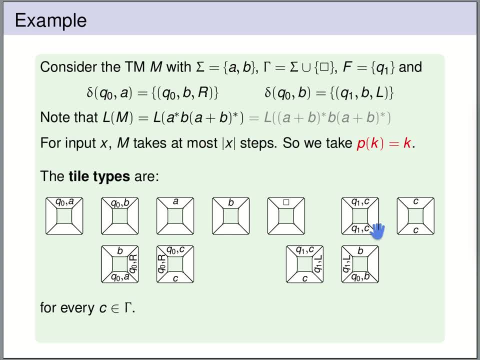 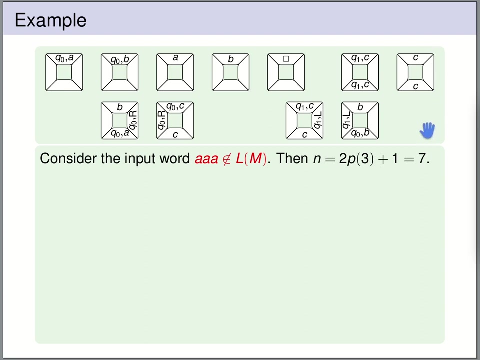 have any letter C of the tape alphabet. we can just copy Q1C to Q1C. So as soon as we reach an accepting state Q1, we can finish the tiling by simply copying. Now we have these tile types And we want to reduce the question whether the word AAA is in the language of the word. 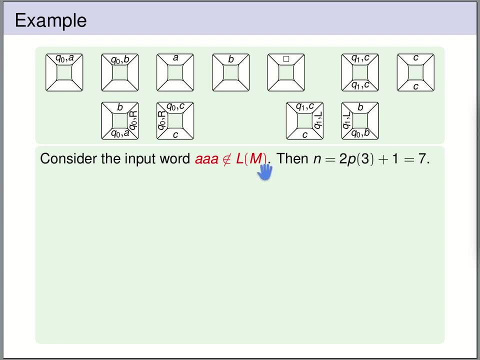 And yes, it is And it is – so we are sending it to our boundary totally curved. We're going to get it to it by forcing its will from the language of the Turing machine to the bounded tiling problem. Now we choose, as size of our bounded tiling problem 2 times P of the length of input word 3, so 2 times p of 3 plus 1.. So the size of our bounded tiling problem is 7 times 7.. We start with the first row that has only blank symbols. to the left of the middle We have the distance심ple choreography and then one of your simple Colin Williams symbols. 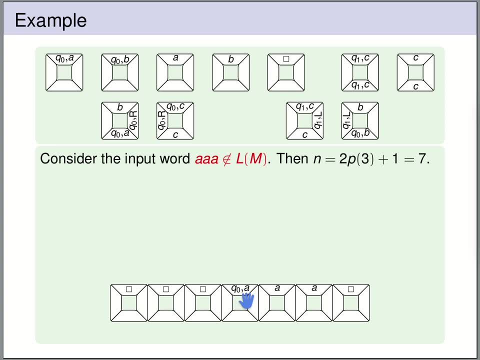 Now let's see how it would work. Here I have the Ziat on. our Finlay is the hasn inичноざ Coffee protector. All right, so this is 1.. When I add this final state, I, We have, starting at the middle, the input word. so we have AAA on top. 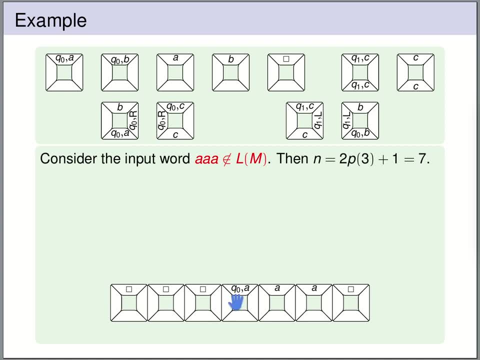 Only at the first letter of the input word we have our state Q0, because that's the starting state of our Turing machine and that's the place where the head of our Turing machine stands in the beginning. And in order to have three cells to the right of the head, we add one additional blank symbol to the right of our input. 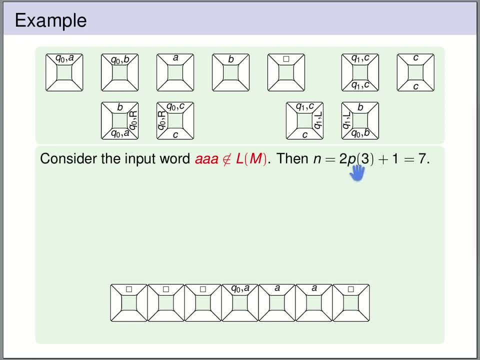 We have to make sure that we have P of three cells to the right of the middle. So in total we have a starting row of seven tiles. Now how can we tile here What fits on top? On top fits these tiles. here We have a Turing machine in state Q0, we read an A. 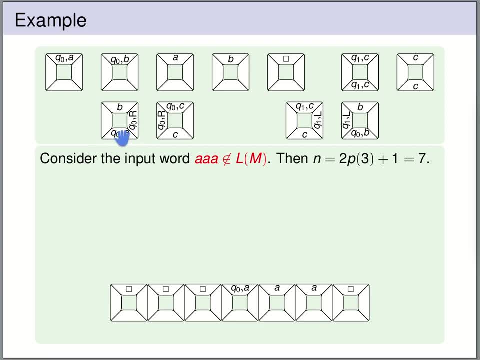 So we have a Turing machine in state Q0, we read an A. So we have a Turing machine in state Q0, we read an A, So we can put this tile on top, and that means that we have to put this tile next to this. 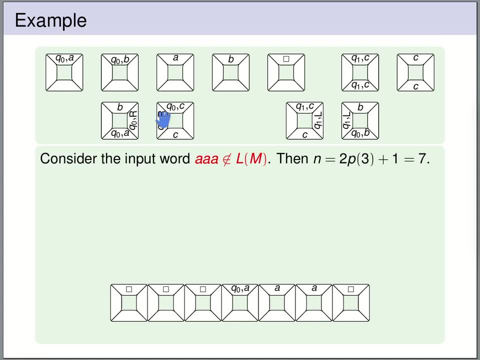 This is the only one that matches horizontally And the C here is in this case an A, So we put this tile on top here, where the C is instantiated by A, And for all other tiles we simply copy the tape. We use these tiles. 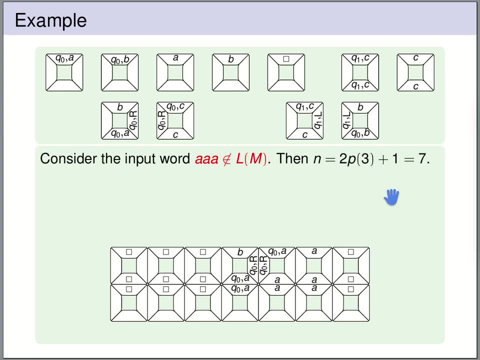 That we have for any C in the tape alphabet, to simply copy the blank symbol, copy the A, copy the blank symbols through here And now we see that indeed, we have simulated one step of our Turing machine. We were in state Q0, we are reading an A. 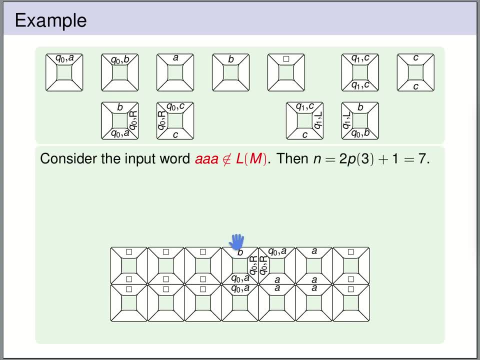 The A has now been overwritten by a, B. We have moved to the right, still in state Q0. And we are now standing on this A. Now again, what can we put on top here? We still have a Q0, A. 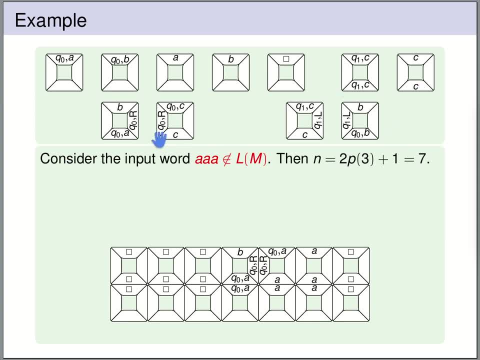 So these tiles don't match, this doesn't match. So the only thing we can put on top is again this tile, and again to the right of it. we must have this tile, because nothing matches horizontally. And again the C is instantiated by an A. 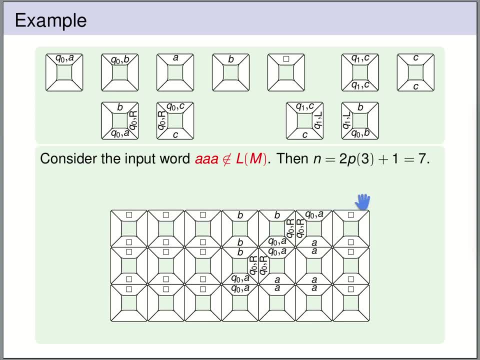 So we put the same things on top. We again copy here and we copy everything here. So we have again overwritten by an A. So we put the same things on top. We again copy here and we copy everything here, Overwritten the A by a, B. 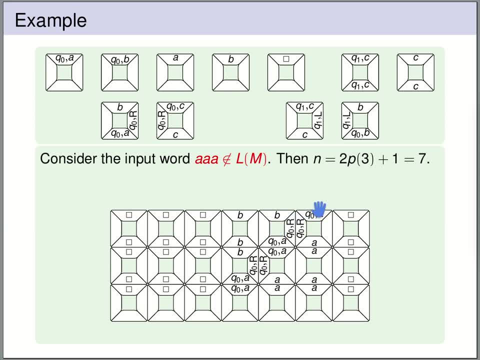 We have moved one step to the right. So now the Q0 stands on the last input letter A here. What can we put on top here Again for Q0, A? we don't have a choice. We have to use this tile. 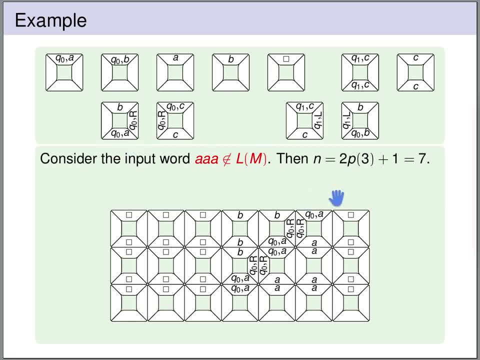 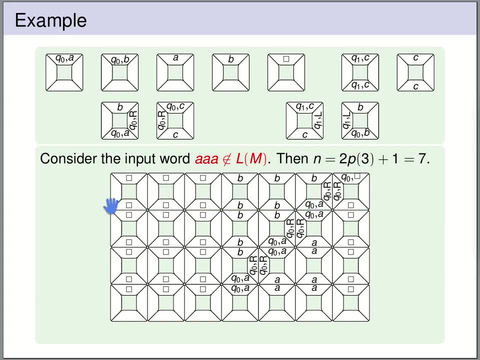 Now the C here is a blank symbol And everything else we copy And everything else we copy. So now we are having a tile here with on the top color Q0 blank. So now we are having a tile here with on the top color Q0 blank. 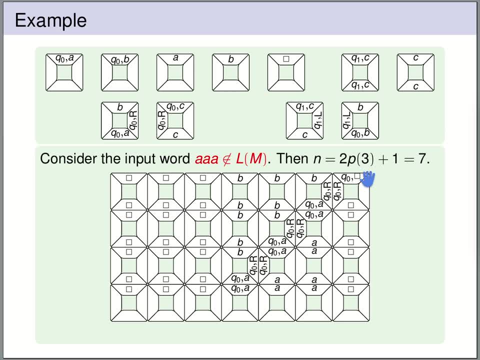 So now we are having a tile here with, on the top color Q0 blank, And for Q0 blank there is simply no matching tile. And for Q0 blank there is simply no matching tile. And for Q0 blank there is simply no matching tile. 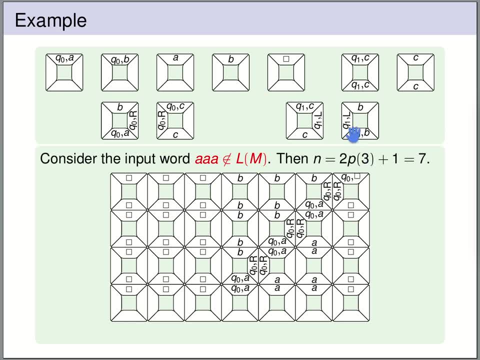 So we cannot go on from this. We cannot continue tiling. There is no way to put anything on top here. There is no way to put anything on top here. So this is non-complete tiling and there is no way to complete it. 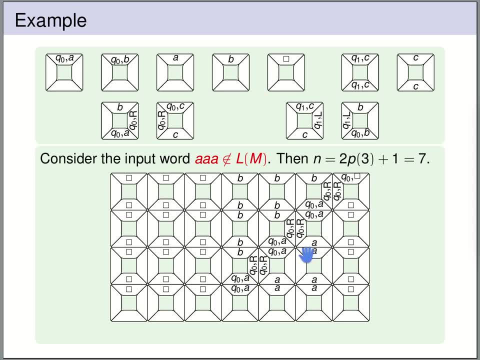 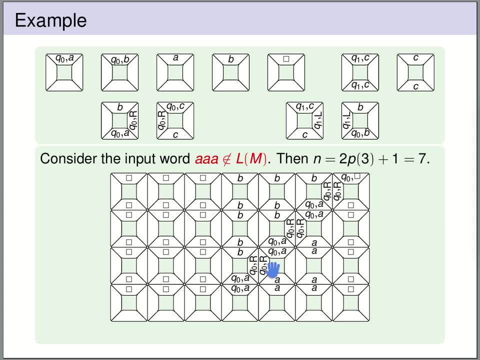 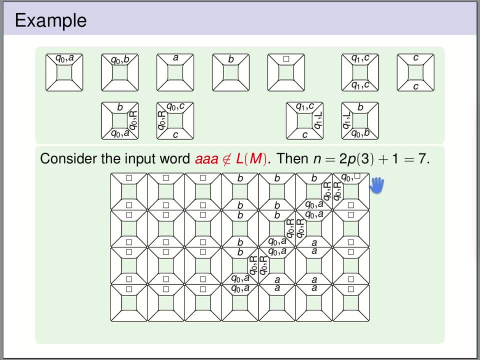 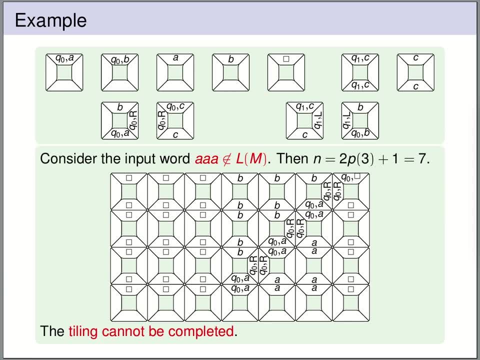 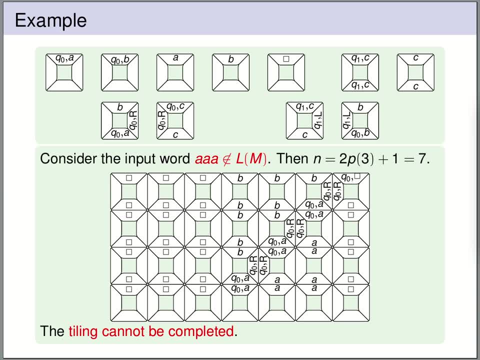 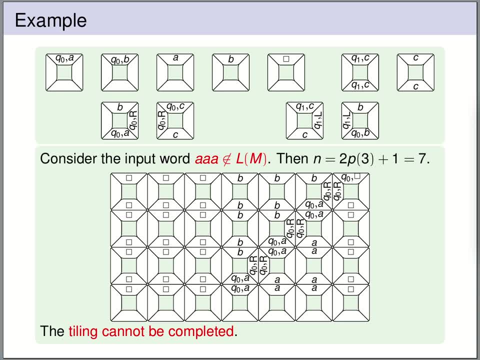 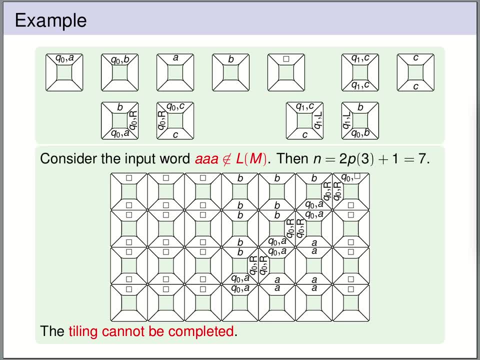 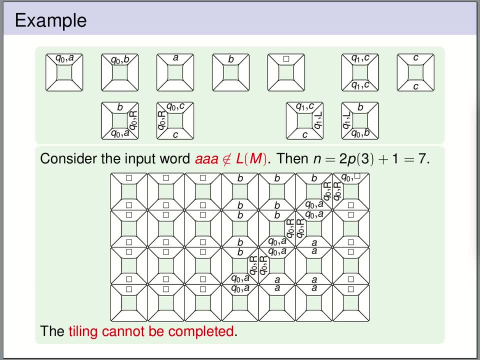 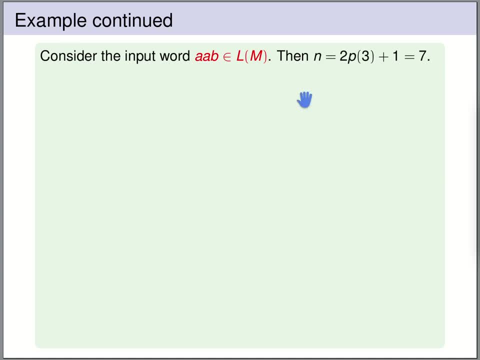 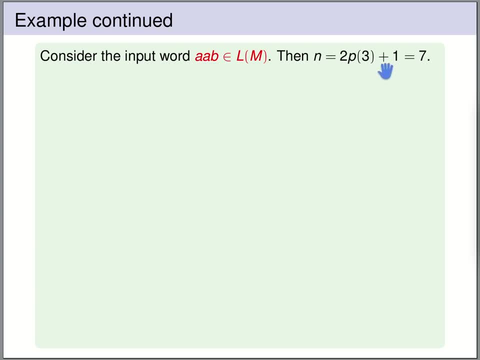 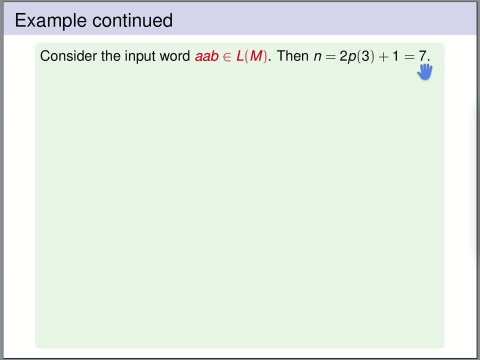 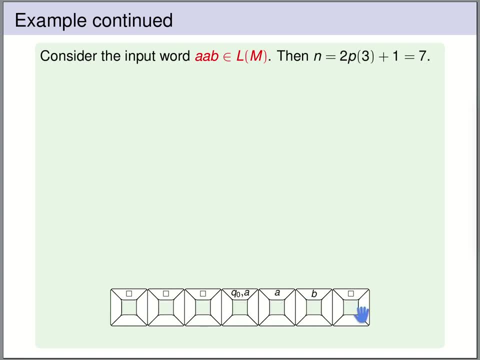 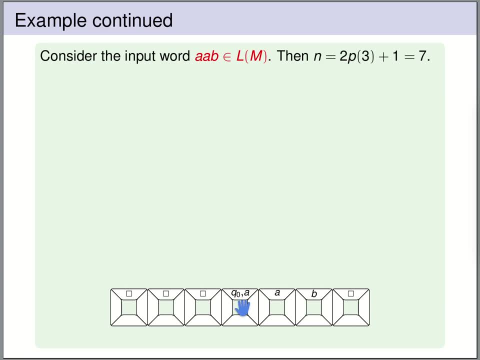 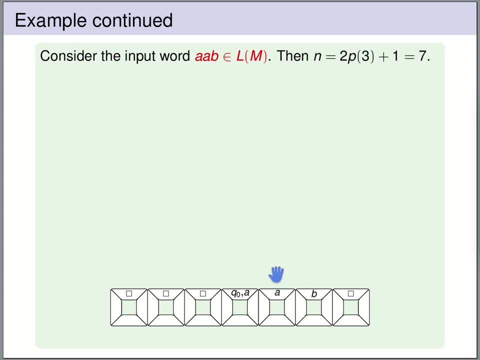 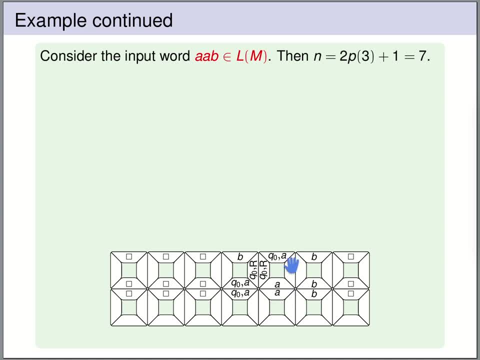 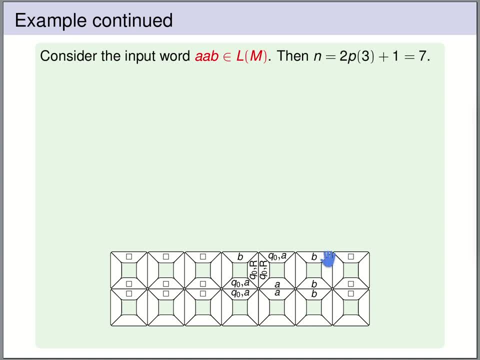 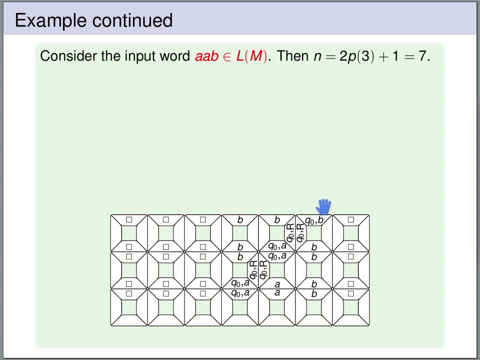 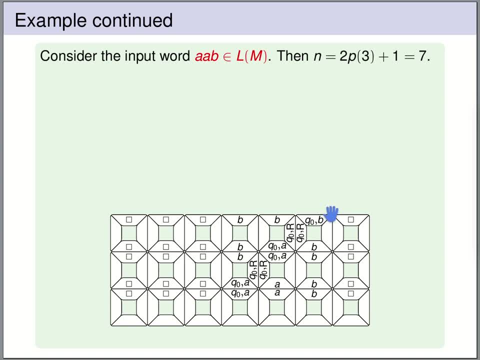 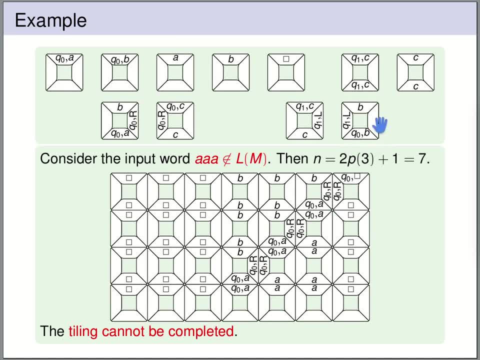 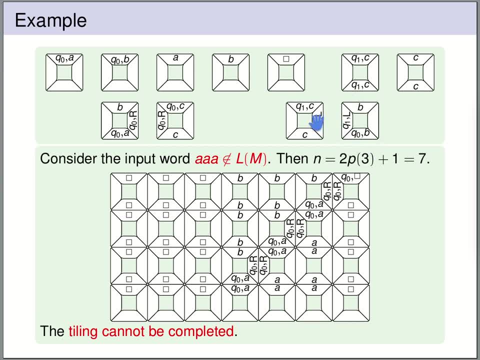 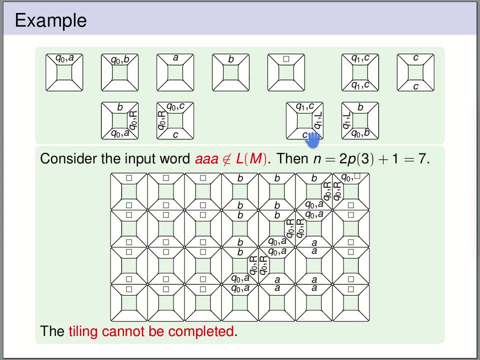 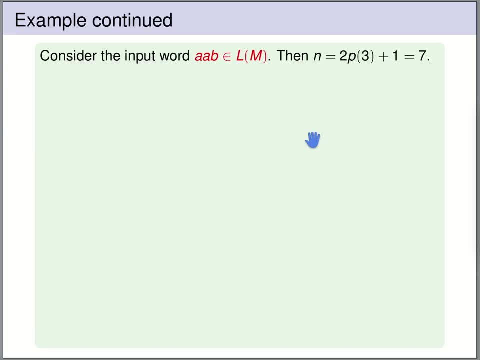 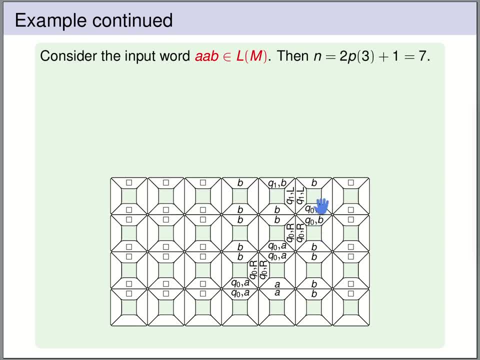 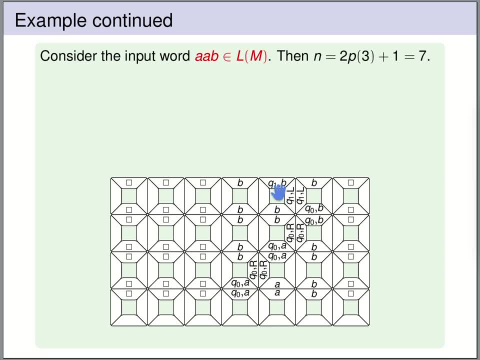 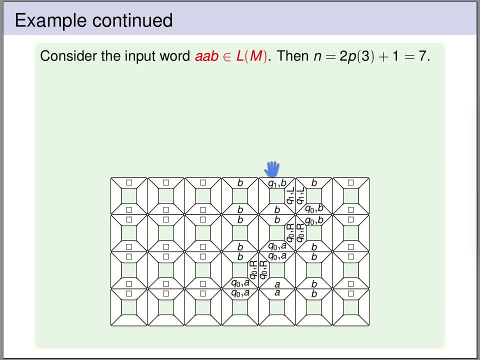 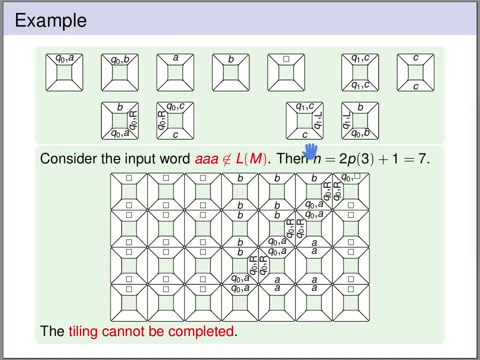 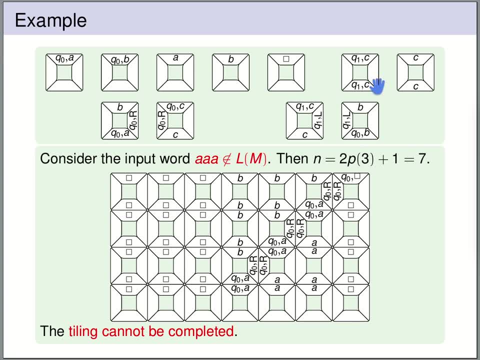 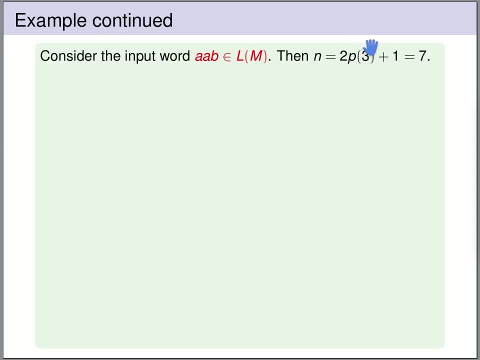 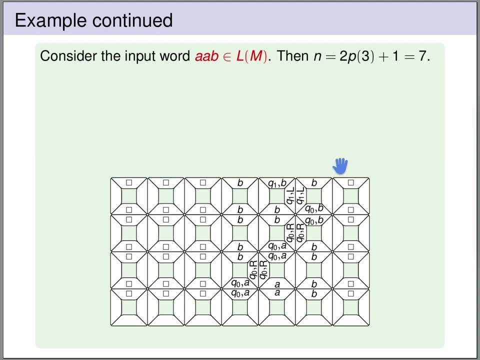 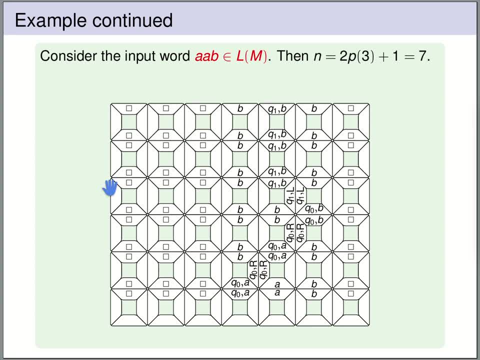 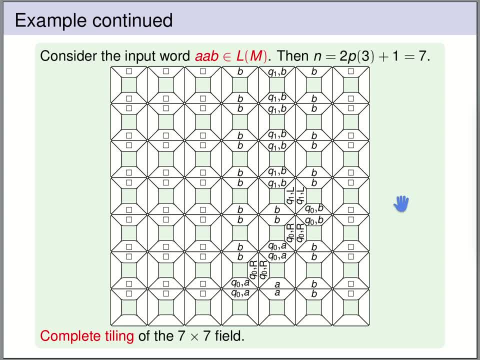 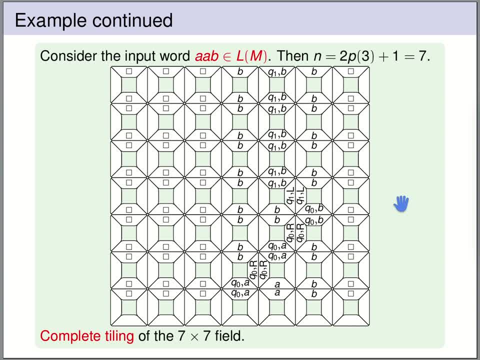 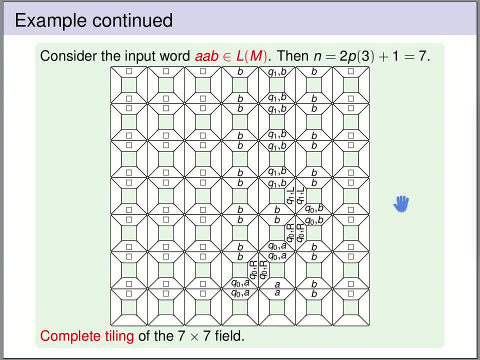 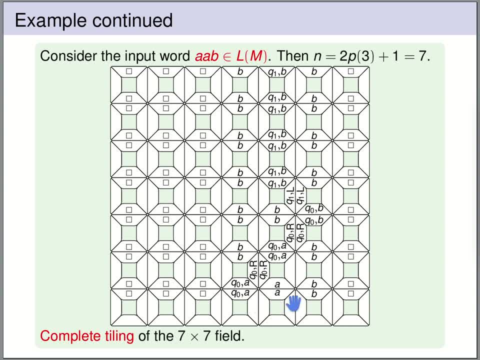 So this is non-complete tiling and there is no way to complete it. So this is non-complete tiling and there is no way to complete it. So we have reduced the question about membership of words in the language of the Turing machine. 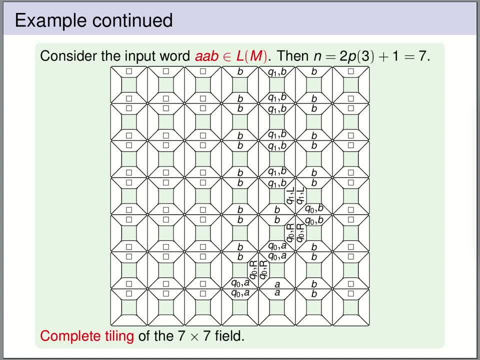 to instances of the bounded tiling problem and the translation from a word to a bounded tiling problem is polynomial. we have only polynomial many tiles and the polynomial size of the start row. So this means that we have a polynomial reduction from the membership question to the bounded 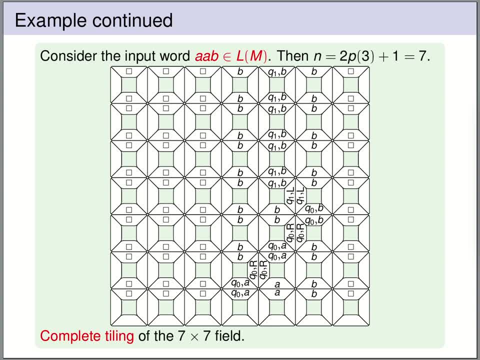 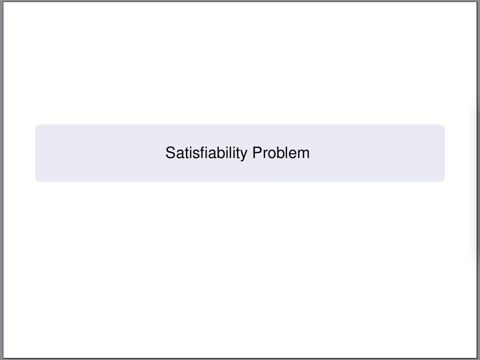 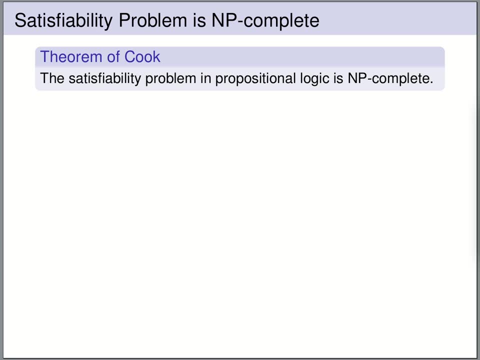 tiling problem. So we now know that the bounded tiling problem is NP-complete and we are going to use it to show that also satisfiability in propositional logic is NP-complete. We have already discussed that the satisfiability problem in propositional logic is in the class NP. 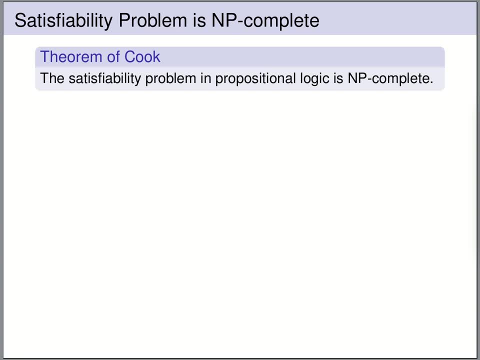 We are now going to show that it is NP-complete, so that every other problem in the class NP can be reduced to it in polynomial time. In order to prove this, it suffices to show that some NP-complete problem can be reduced in polynomial time to the satisfiability problem. 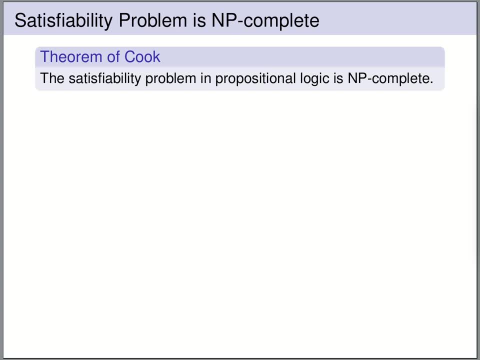 And we are going to use the bounded tiling problem. We've just seen this And we know that the bounded tiling problem is NP-complete, So it suffices to show that there is a polynomial time reduction from the bounded tiling problem to the satisfiability problem. 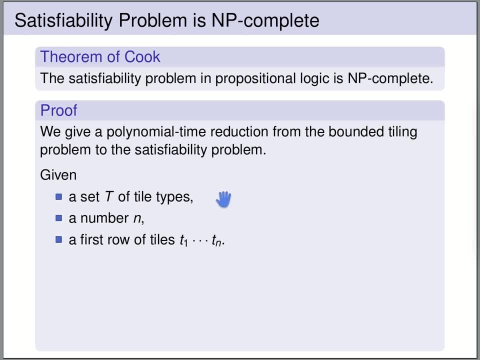 So we start with an instance of the bounded tiling problem. We have a set T of tile types. Each of these tile types we can use arbitrarily. often We have a number N. That's the size of our tile. That's the size of our bounded tiling problem. 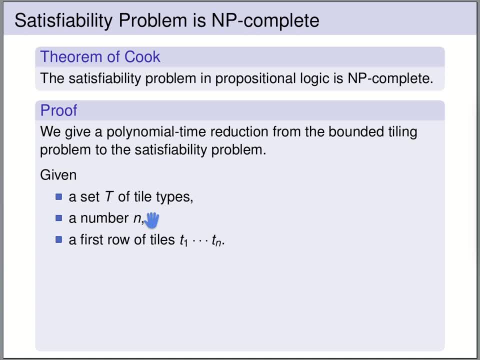 That's the size of the field that we work on. So it's a square field. N times N And we have given a first row. The tiles in the first row are T1 up to TN. So how are we going to create a propositional logic formula now? 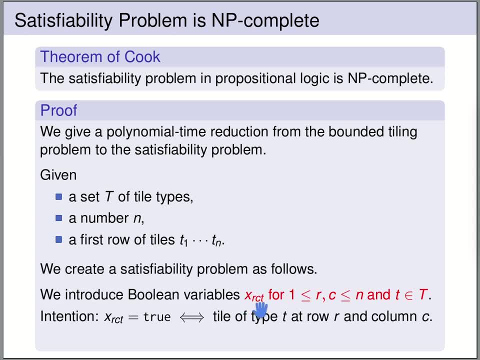 We introduce Boolean variables of the following form: X, R, C, T. R represents a row number, So it ranges between 1 and N. C represents a column number, It ranges between 1 and N as well, And T is a tile type. 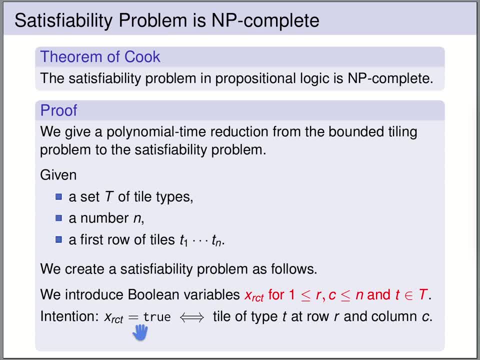 The intuition is that this Boolean variable will be true if, and only if, at row R in column C we have a tile of type T. So we have to create formulas that make sure that this intuition is indeed true and that the tiling is correct. 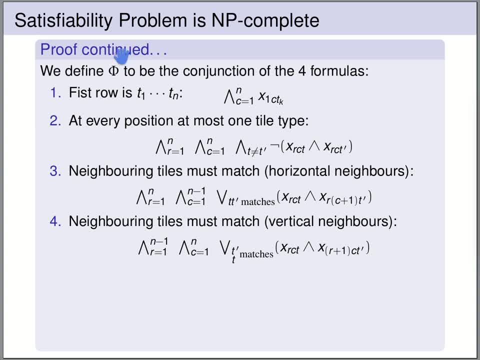 So we translate our bounded tiling problem into a formula phi, And this formula phi is the conjunction of the four formulas shown on this slide. So let's have a look at each of these formulas. The first formula expresses that the set is equal to 0.5 times N because the form is equal. 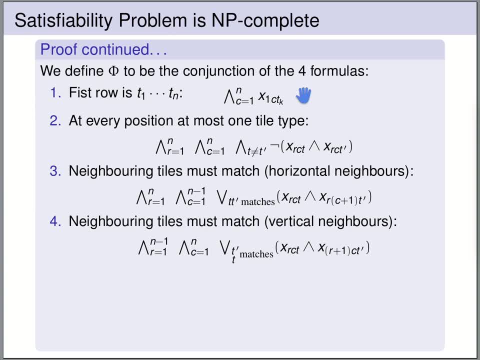 to 0.5.. starting row must be correct. So it says: for every column c, from 1 up to n, the tile in row 1 at column c must be the tile tk And tk is the kth tile of our starting row. The second formula says: 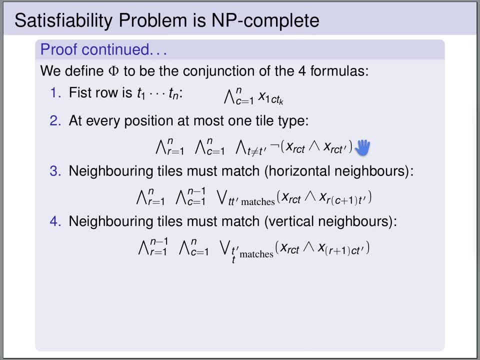 that we never have two different tiles at the same position. So, for every row r, from 1 to n, for every column from 1 to n, for each distinct assignment of tile types t, t' we do not have the tile t at row r, column c, and, at the same time, the tile t' at row r and column c. 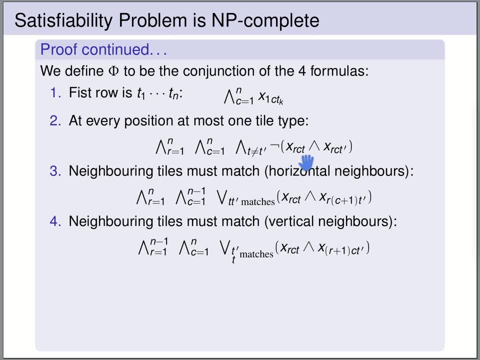 So we never have at the same position two different tile types t and t'. The third formula says that we never have two different tile types t and t'. The fourth formula says that at every position in our field we must have horizontally matching tiles. So for every row, from 1 up to n, for every column, from 1 up to n-1, and here we only go up. 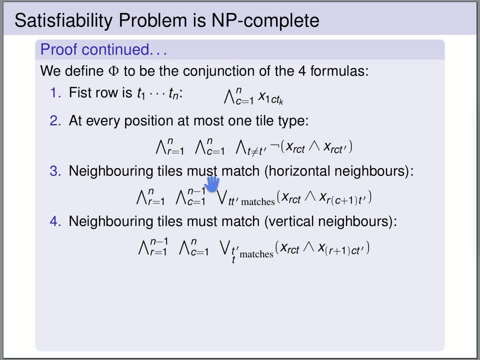 to n-1, because we want to look at the right neighbor. This big disjunction here says that one of these formulas has to be true. So there has to be one assignment of horizontally matching tiles. So we have to have one assignment of horizontally matching tiles. So we have to have 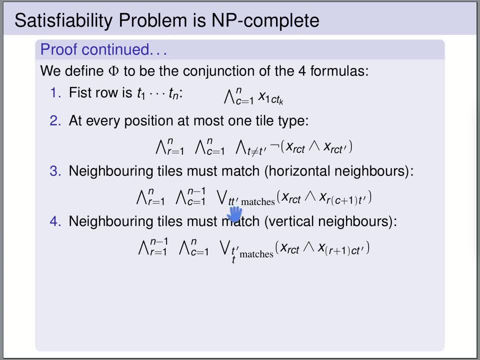 one assignment of horizontally matching tiles t and t' fitting horizontally next to each other such that at the position row r and column c we have tile t and at its right neighbor, so row r and column c plus 1, we have tile t'. 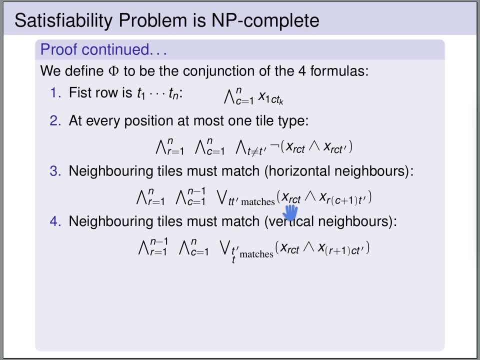 So for the position rc in our field we have some assignment of horizontally matching tiles- t, t'- So it has to match with its right neighbor. And the fourth formula says the same, but for vertically matching tiles. So for every row from 1 up to n-1,, for every column from 1 to n. 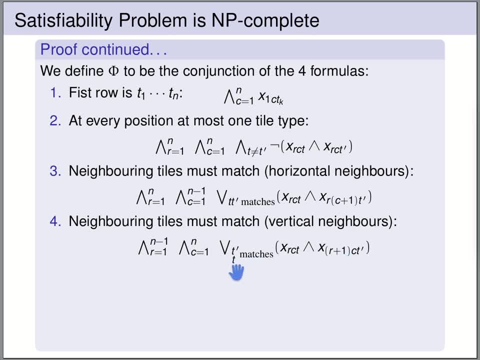 there must be some assignment of vertically matching tiles, so t and above it t', such that at row r in column c we have tile t and above it, in row r plus 1 and column c, we have tile t' So the first formula makes sure that the starting row is okay. The second makes sure that we never. 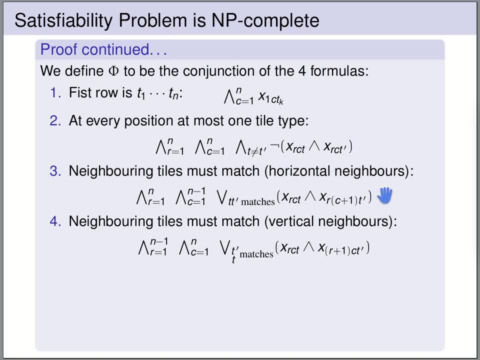 have two tiles at the same position. The third makes sure that horizontally the tiles match, and the fourth makes sure that vertically the tiles match. If we put all of them together in one conjunction then we achieve that. the formula phi is satisfiable. 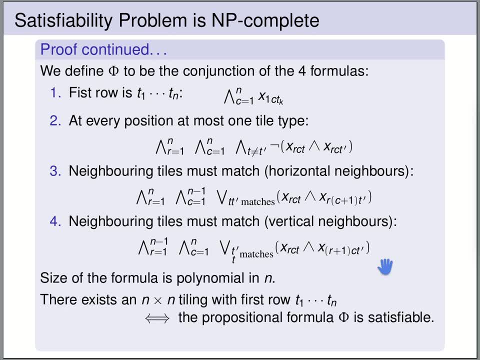 If, and only if, the bounded tiling problem has a solution And indeed we have a polynomial time reduction from the bounded tiling problem to formulas in predicate logic, because our formula phi has polynomial size with respect to the size of the bounded tiling problem. So here we have linear size in n, here we have n squared times. 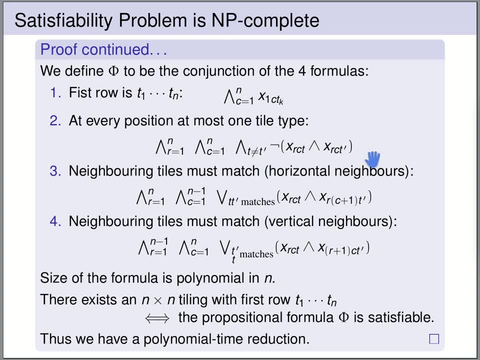 the number of tiles squared, still polynomial. Here we have also n squared times the number of tiles squared and the same here. So the size of the formula that we construct is polynomial in the size of the bounded tiling problem. Let's have a look at an example. We are going to reduce this equation by the number of the tiles. 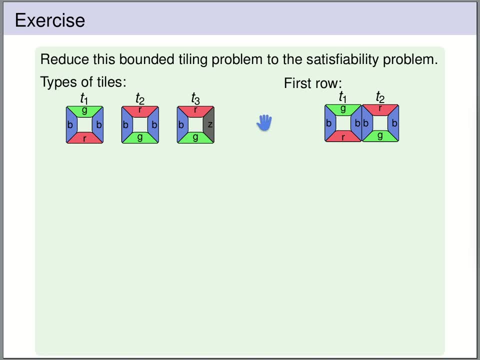 instance of the bounded tiling problem, to a satisfiability problem. Here we have given three tile types: T1, T2, T3, and we are given this first row. so our first row consists of tiles T1, T2.. Now we translate it into a formula in propositional logic as follows: 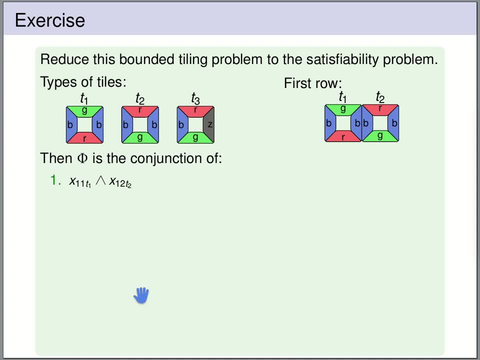 The formula phi will be the conjunction of four formulas. The first formula expresses that the first row is T1, T2.. So we say that the variable X11, T1 must be true. so this says: on our field, at position, we have the tile T1.. So in row 1, in column 1, there's 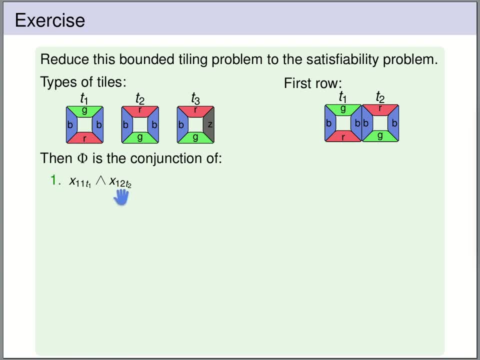 tile T1.. Also X12, T2 must be true. So in row 1, column 2, we have tile T2.. So this expresses in the first row we have tiles T1, T2.. The second formula expresses that at no position on our field we have two different tiles. 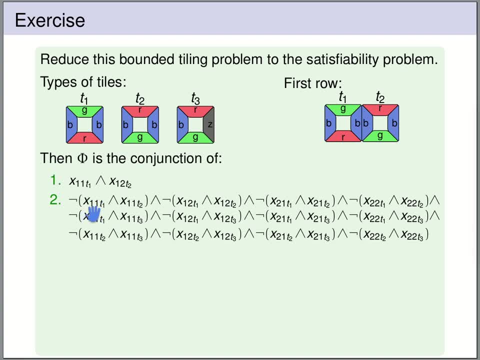 So at position we do not have at the same time, we do not have at the same time tile 1 and tile 2. So when we have two tiles, one at the time We have T1 and T2. 2. The same for position 1-2, 2-1 and 2-2. We never have tile 1 and tile 2 at these positions. 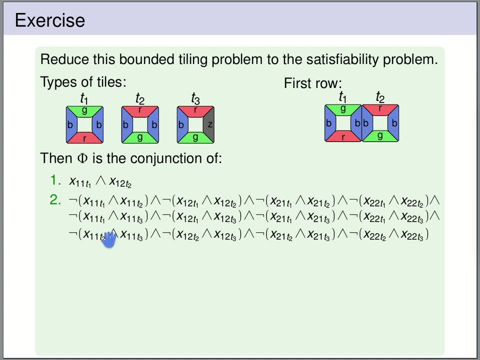 at the same time. Then we need the same for tile 1 and tile 3.. So we do not have tile 1 and tile 3 at the same time at position 1-1.. The same for position 1-2,, 2-1 and 2-2.. And finally we have 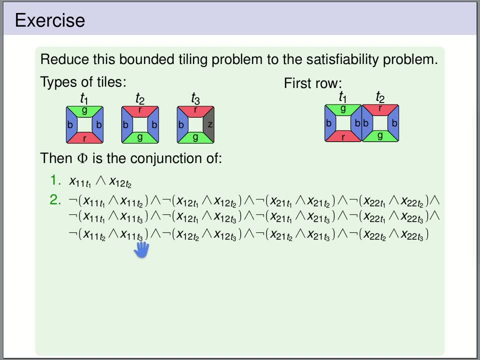 to express that we never have tile 2 and tile 3 at the same position, Neither at position 1-1,, 1-2,, 2-1 or 2-2.. So, putting all these together, we have expressed that we never have two different. 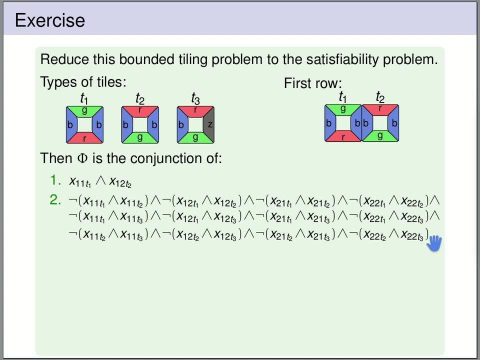 tiles at the same position. Now the third formula expresses that at every position we must have horizontally matching tiles. So we look first at the position 1-1 and the tile at position 1-1 must match with the tile to its right, So with the tile at the position 1-2.. So this is this upper two rows here. 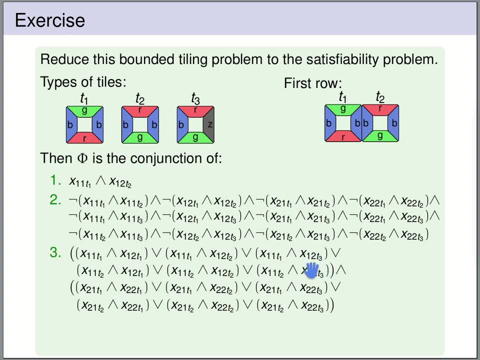 This first two rows. they express that the tile at position 1-2 and 1-1. they must fit together horizontally. So what tiles fit horizontally together? T1 can be on the left and T1 can be on the right. We have blue on the right side so we can have another tile, T1, right of it. They would fit. 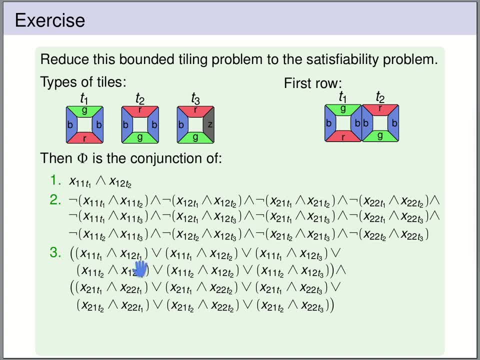 horizontally, So T1 and T1 could be next to each other, Or we have T1 and T2.. They also fit together. We have blue, So T1 could have T2 right of it, Or T1 could have T3 right of it. 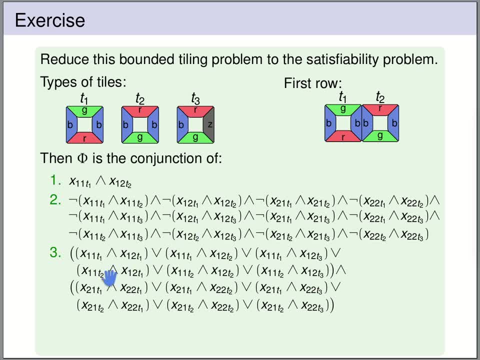 Because here is blue and here is blue, Or we have a tile, T2 and T1 right of it. T2 can have on the right side T1.. T2 can have on the right side T2 also. T2 can have T2 on. 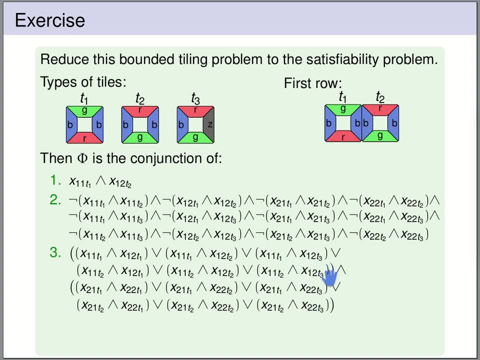 the right, And T2 can have T3 right of it. T2 can have T3 right of it. T3 cannot have anything right of it. So these are the only combinations: T1, T1.. T1, T2.. T1, T3.. T2, T1.. T2, T2. And T2, T3.. One of these must be true, So we 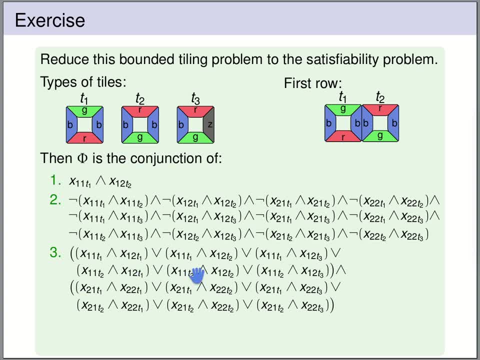 have a big disjunction. One of these combinations must be true. And then the second two rows. so these two rows, they express the same property. but now for the horizontally connected tiles at positions T1, 1 and 22. So its exactly the same. 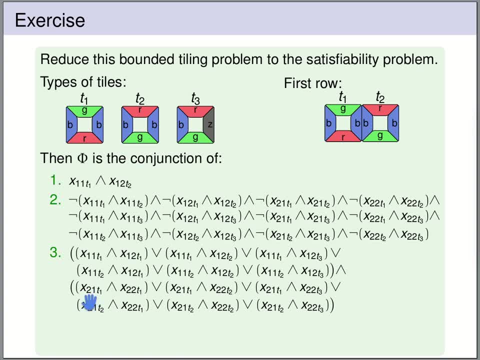 But now, instead of positions 1, 1, 1, 2, at positions 2, 1, 2, 2.. So the second row. So this formula expresses that all tiles fit horizontally nicely together, so that the connected sides have the same color. 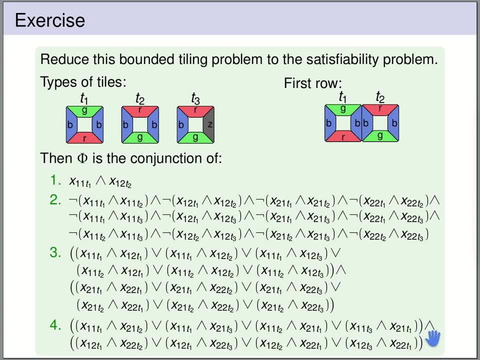 And finally, we have a formula that expresses that the tiles fit vertically, Vertically, vertically together, so that the connected sides of tiles that are vertically above each other have the same color. so here we say that the tile at position 1, 1 should match with the tile at 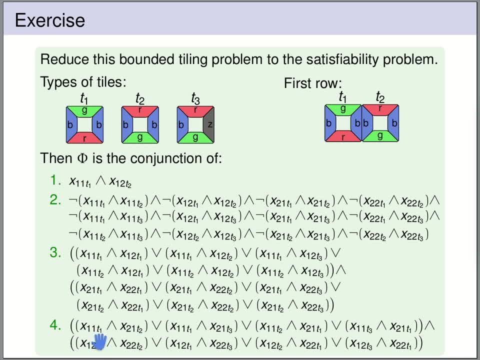 position 2: 1. so at position 1: 1 we could have tile t 1, and then above it could be on the top we have green, so above it could be either t 2 or t 3. it's expressed here. if we have at position 1: 1, we have. 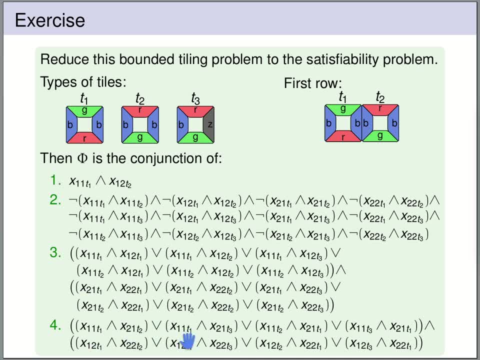 t 1, then we can have t 2 above it. or if we have t 1, then we can have t 3 above it. or we can have at the bottom t 2 and then we have red on the top, so above it can only be t 1. if you have t 2, then 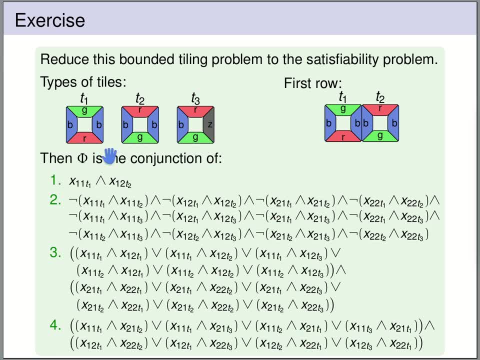 above it can be t 1, and likewise if you have t 3, then above it can only be t 1. so this first row here expresses this for the left column, so for column 1, 1 one. and then the second row expresses the same thing, but for column two. 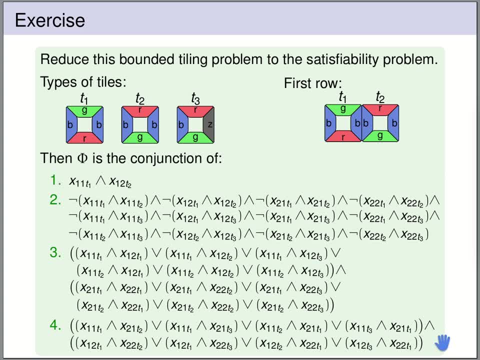 So if we put all these formulas together in one conjunction, then we express that we have a correct solution of our bounded tiling problem and it holds that the bounded tiling problem has a solution if, and only if, this formula is satisfiable. 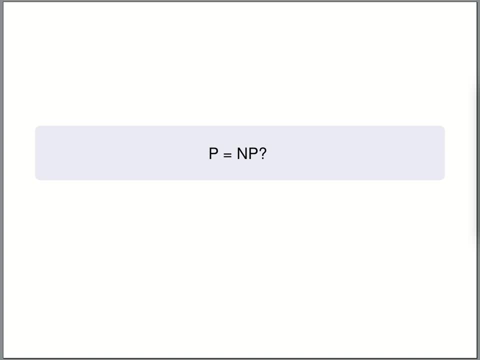 Let's have a look at the famous question whether P is equal to NP. If there would be an NP-complete problem, L that is also in P, then it would immediately follow that P is equal to NP. So if some NP-complete problem is solvable in deterministic polynomial time, it follows: 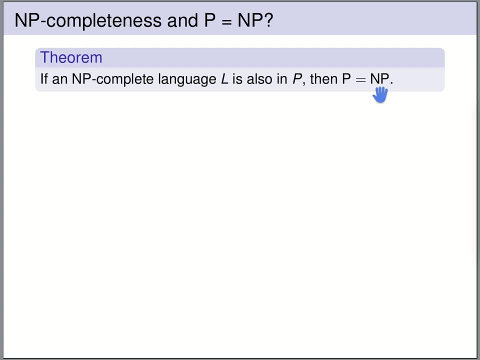 that all problems in NP are solvable. And did the police Escape deterministic polynomial time? Let's prove that. So let's assume that we have such an NP-complete problem, L that is also in P. Now we show that all other problems in NP are also solvable in. 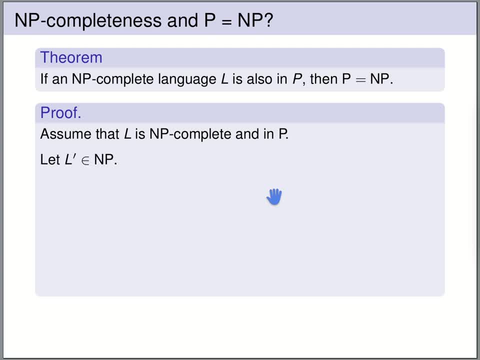 deterministic polynomial time. So let L' be some problem in NP. Since L is NP-complete, we know that L' can be reduced to L via a polynomial time reduction. So we have some polynomial time reduction, F, such that a word is member of L' if, and only if, the F image of this word. 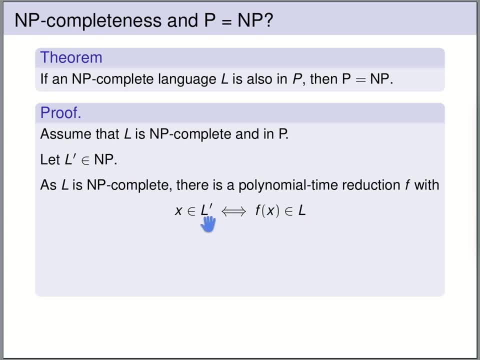 is a member in L, So X is a member of L' if, and only if, F of X is in L. Now, by assumption, L is L' In P, so we can check whether F of X is in L in deterministic polynomial time. 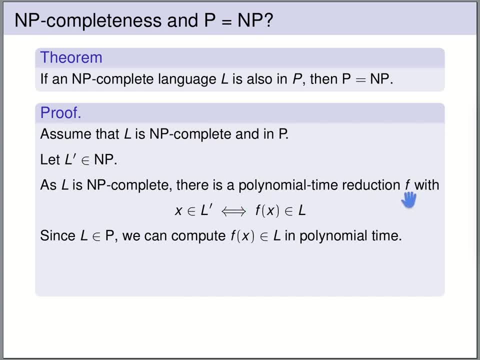 Moreover, we have a polynomial time reduction F. So in order to check whether X is in L' we simply compute polynomial time reduction F and then we check membership in L in polynomial time. So we have two polynomial time reductions. So we want to know the value of membership for each detector graph. 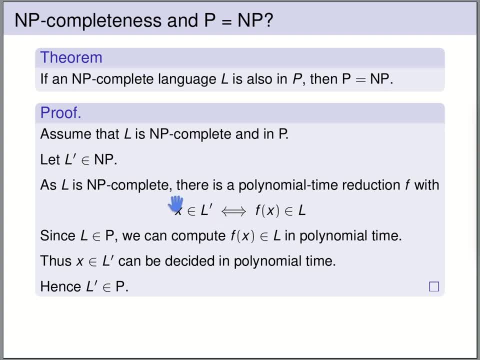 Let's look at item at point, for example now. And if F of X is in P, okay, we decide that it can. E is an integer. If F is in L, we would generally say that P is in Np and if the yanlış answer is correct. 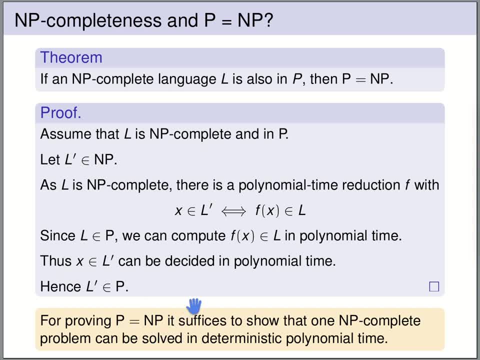 that's correct. So on representative time, let me take a look at this. We were given a row right And then we can actually use this in polynomial time procedures. Next, the combination of the two is again polynomial time, So we can decide membership in L' in polynomial time, And that means that L' in P, nex Worth is in P. 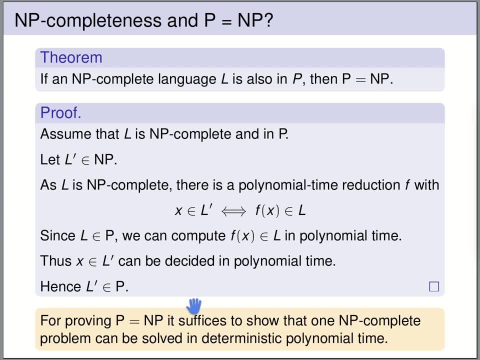 and show that it is NP. So take your favorite NP complete problem and find a deterministic polynomial time algorithm for it. In principle, that's all that is needed, and then it would be clear that the classes collapse. both are the same. Of course, this is not that easy. As I said before, 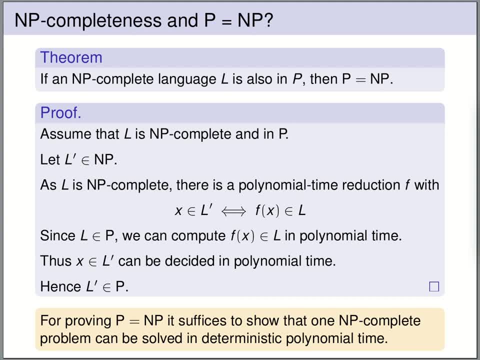 this is probably at the moment the most famous open problem in computer science. So finding a deterministic polynomial time algorithm for some NP complete problem is really really difficult and probably even impossible if the classes are not the same. Let's have a look at the complexity class co-NP. 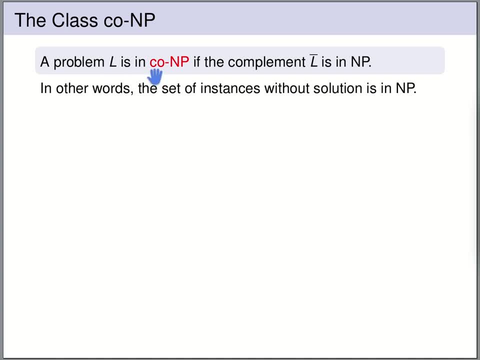 A problem, L is said to be in the complexity class co-NP. if the complement is the same, The complement of L is in the complexity class NP. So in other words, the problem is in co-NP if the set of instances of the problem for which the answer is no is in NP. 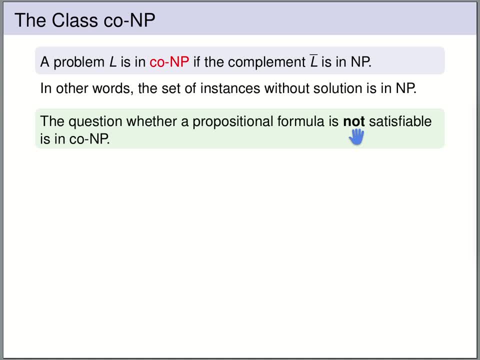 So, for instance, the question whether a formula is not satisfiable is in co-NP. It's unknown whether NP and co-NP are the same, So in particular, it's unknown whether the satisfiability problem itself is in co-NP. So we know the satisfiability problem is in NP and the question whether a formula is not. 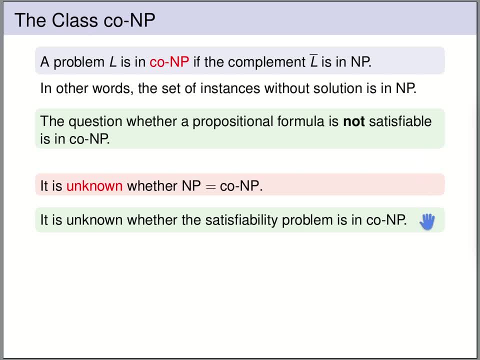 satisfiable is in co-NP. but whether the satisfiability problem is in co-NP is unknown. The problem is, if you want to show that the formula is not satisfiable, it doesn't suffice to simply guess some assignment. We have to show that the formula evaluates to false for all. 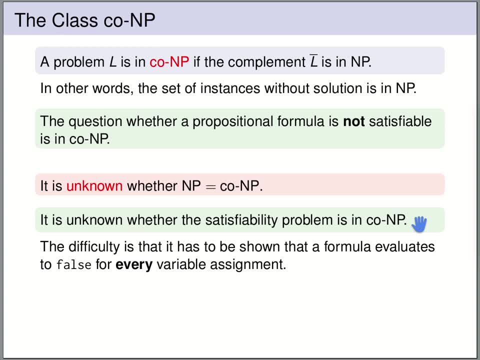 assignments. And the question is: how do you do this with polynomial time guessing? If there is some NP complete problem that is in co-NP, then the two complexity classes, NP and co-NP, coincide. There are problems known that are in co-NP and co-NP that are in co-NP. 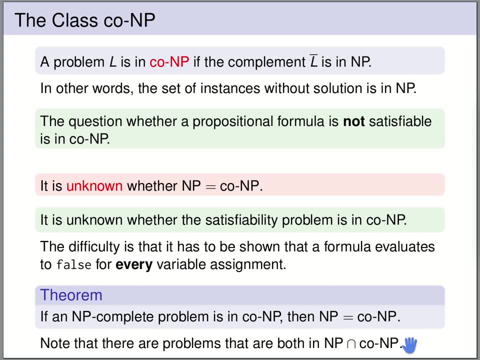 There are problems known that are both in NP as well as in co-NP, And for many of these problems, at some point polynomial time deterministic algorithms are found. So for many of these problems it has turned out that they were not only in the intersection of NP and co-NP, but they were actually in P. 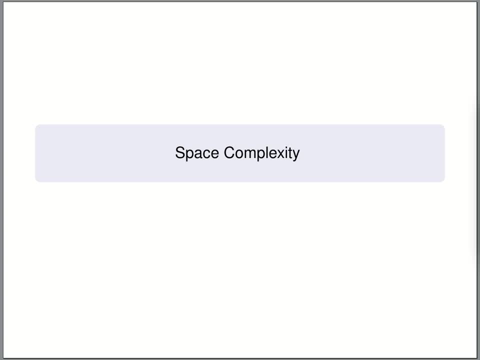 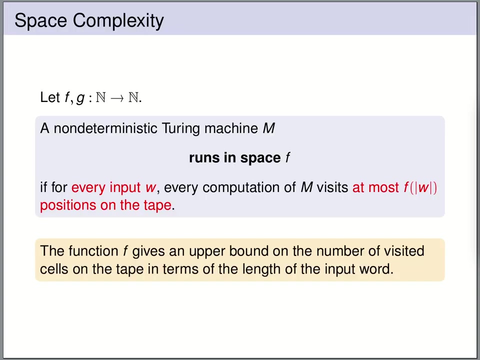 So far we've looked at time complexity. So how much time does a computation take? But next to the time that the computation takes, it's also interesting to look how much space, how much memory is needed for a computation. F and g are again functions over the natural numbers. 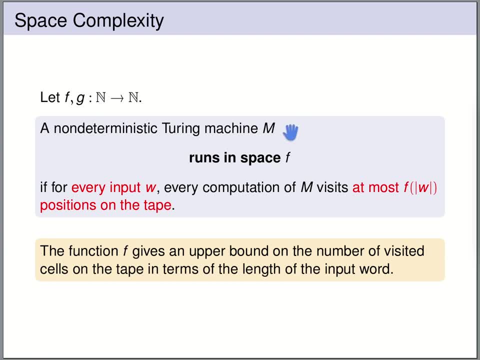 We say that a non-deterministic Turing machine runs in space f if for every input word w, W, every computation of the Turing machine visits at most f of the length of W position on the tape. So this function f gives an upper bound on the number of positions that are visited on. 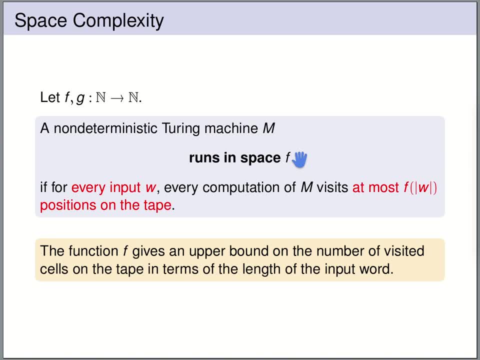 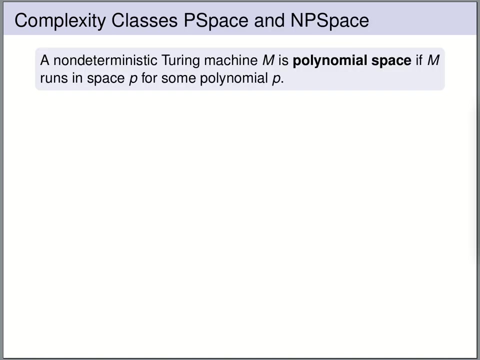 the tape depending on the length of the input word. And this upper bound has to hold for every possible computation of the non-domestic Turing machine. So the function f gives us an upper bound on the memory that is required for this computation. Analogously to polynomial time Turing machines, we can now define what polynomial space Turing 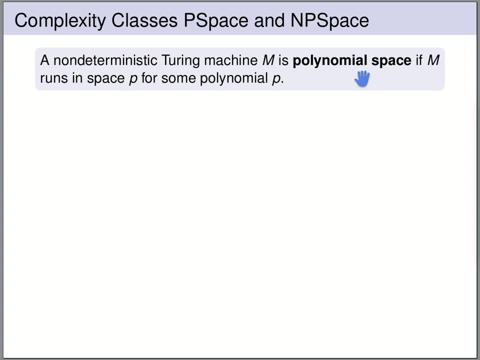 machines are A non-domestic Turing machine. M is said to be polynomial space. if M runs in space, P for some polynomial P. So the function f gives us an upper bound on the memory that is required for this computation. Then we can also define analogues of the complexity classes NP and P, namely NP space and P space. 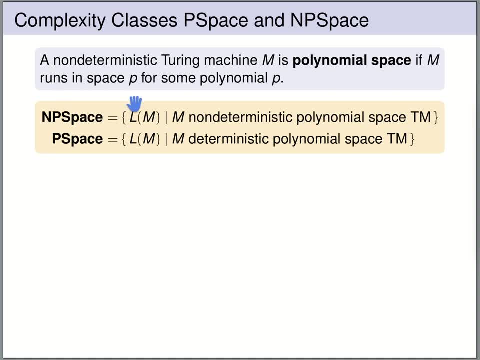 NP space consists of all the languages that are accepted by non-domestic polynomial space Turing machines. P space consists of all the languages accepted by deterministic polynomial space Turing machines. So it's analogous to the complexity classes np and p. for time complexity, but now it's 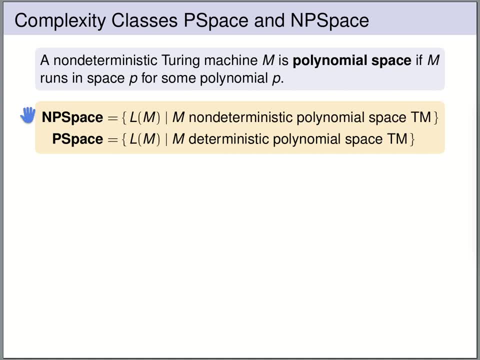 np space and p space for polynomial space complexity, Obviously we have that p is a subset of p space and np is a subset of np space. If we have a Turing machine that runs in polynomial time, then in each time step, in each tick. 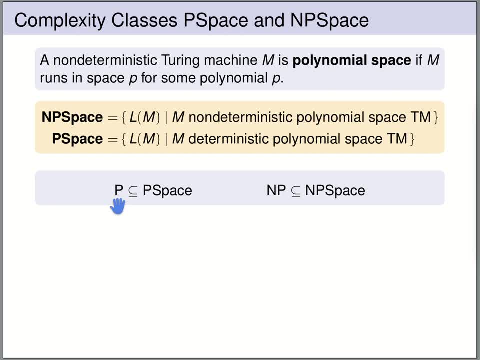 of the clock we can visit only one position on the tape. So if you have a machine that runs in polynomial time, then it can only visit polynomial many places on the tape, And the same for non-doministic machines. Now for the complexity classes p and np. it is not known whether they are the same. 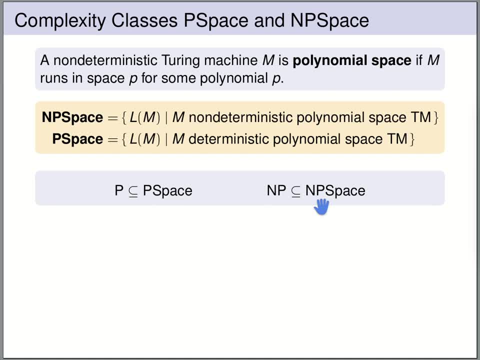 This is the most famous open problem in computer science at the moment. Somewhat surprisingly for the space complexity classes p space and n space, it turns out that the answer is that they coincide. P space is equal to np space. Now the theorem actually says something more general. 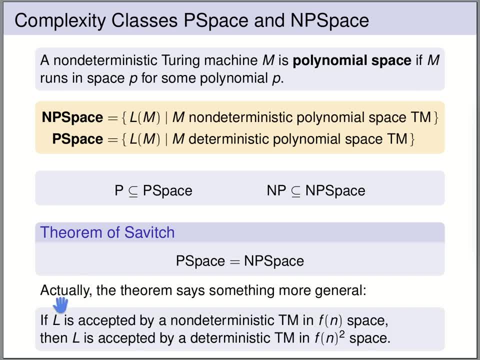 The theorem says that whenever we have a language That is accepted by a non-doministic Turing machine in space f, then this language is also accepted by a deterministic Turing machine in space f squared. So, going from non-doministic to deterministic machines, we need more space, but only quadratically. 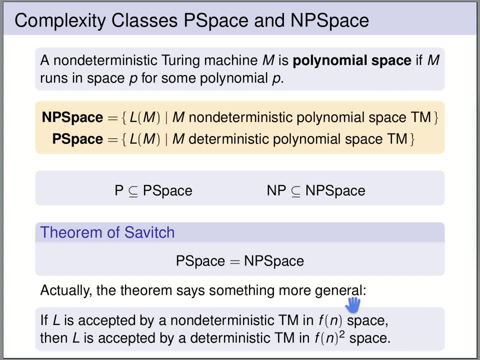 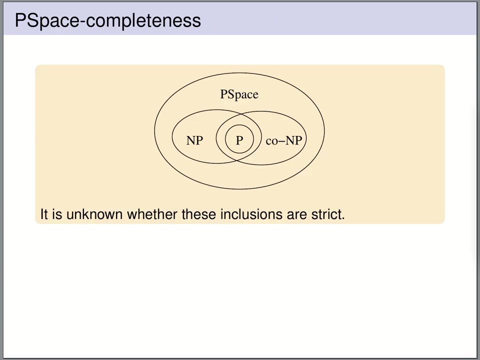 more space. So if we have a polynomial f, Then The square Of this polynomial is again a polynomial. Therefore np space is equal to p space. So this proof of the theorem is actually a very nice construction again. So I suggest you to look into that if you're interested. 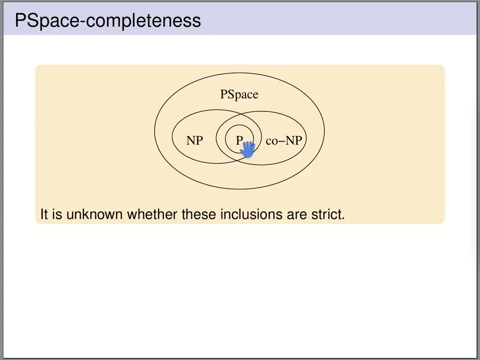 This is a summary of the situation so far. We've seen the complexity class p, That's the class of all the languages accepted by deterministic polynomial time Turing machines. np is the class of all the languages accepted by non-deterministic polynomial time Turing. 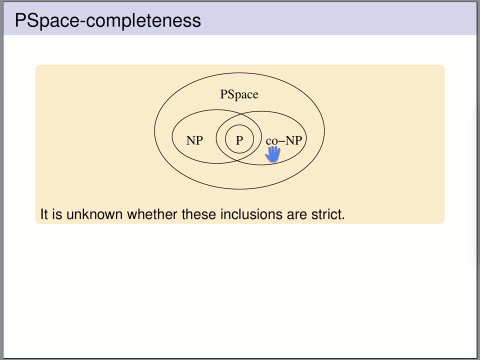 machines. The class co-np consists of those languages for which the complement is in np, And we've seen p space, the class of all the languages accepted by polynomial space Turing machines. For polynomial space, it doesn't matter whether we consider non-doministic or deterministic. 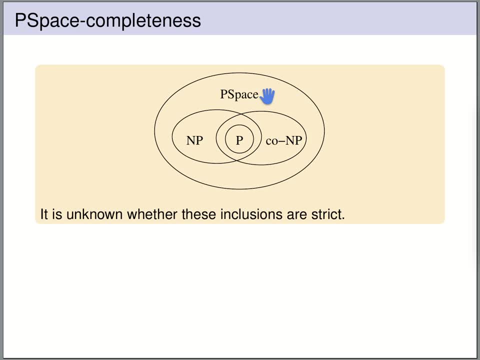 machines. As we've seen on the last slide, the classes p space and np space coincide. Beyond these inclusions, not much more is known. So, in particular, it's not known whether any of these inclusions is strict. It's not known whether p is equal to nP. 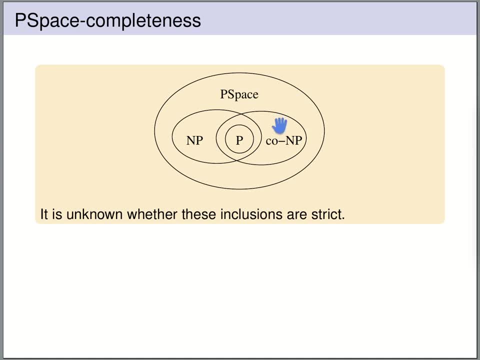 It's not known whether np is equal to co-np And it's not known whether any of these inclusions is strict, So it could be that everything collapses to just P. Analogous to the notion of nP- complete languages. there is also a notion of p- space- complete languages. 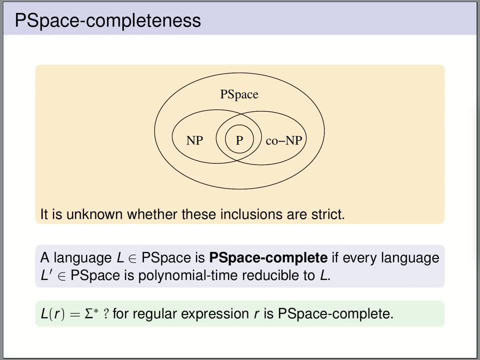 A language L in p space can be taken in any either two ways. The godforsker will recognize that if younaserve becomes a springs Gomez, Then the experiences must be based on two dimensions. What are the two dimensions? Axis is said to be P-space complete if every language L' in P-space is polynomial time reducible to L. 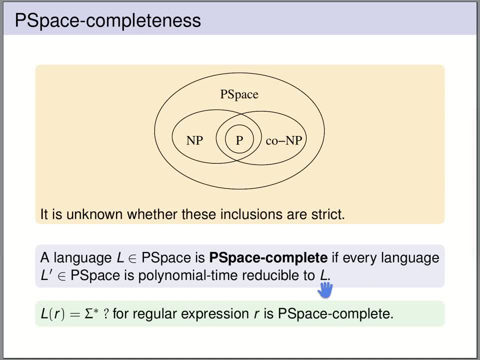 So this definition is absolutely analogous to the definition of NP-completeness. The crucial point here is that, since we are talking about space complexity classes, it is tempting to also use a polynomial space reduction. However, polynomial space reductions are too strong. then they could trivialize the problem If we would use polynomial space reductions. 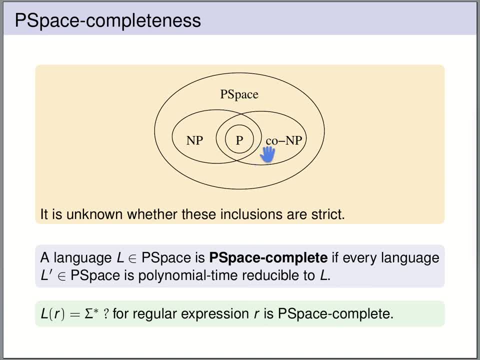 then also problems in P could be P-space complete. That's not what we want, so it's really important that we restrict to polynomial time reductions. An example of a problem that is known to be P-space complete is the question whether, for a given regular expression, R. 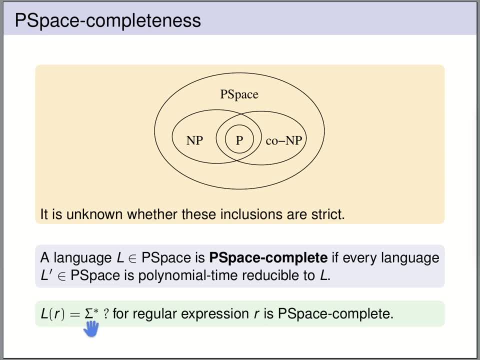 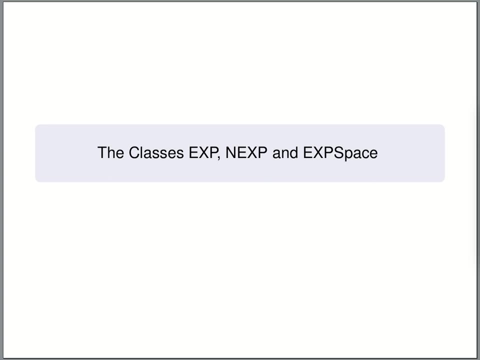 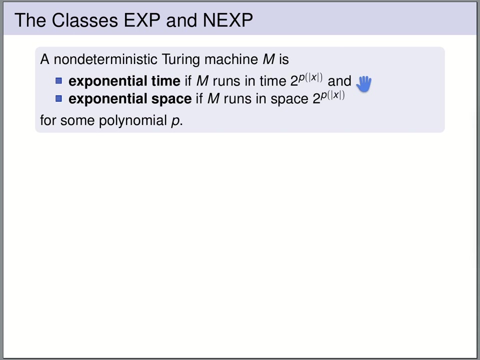 the language of R are all the words over the alphabet sigma. Answering this question is known to be P-space- complete. Analogously to polynomial time and space, we of course also have exponential time and space complexity classes. A non-deterministic Turing machine, M, is said to be exponential time if M runs in time. 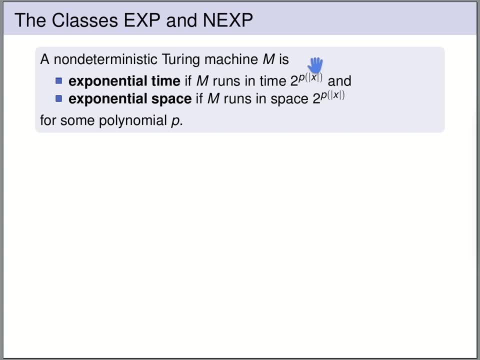 two to the power of some polynomial with respect to the length of the input word. So we have two to the power, P applied to the length of the input word, and P is a polynomial. Likewise we say that the Turing machine is exponential space if it runs in space. 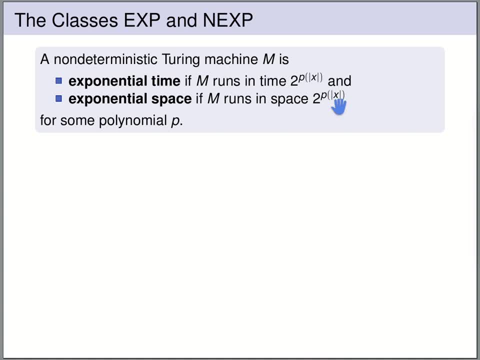 So we have two to the power of a polynomial with respect to the length of the input word. Now, clearly, these are exponential functions. but why did we choose this particular form of exponential function? First of all, in the exponent we have chosen a polynomial, because we do not want to include 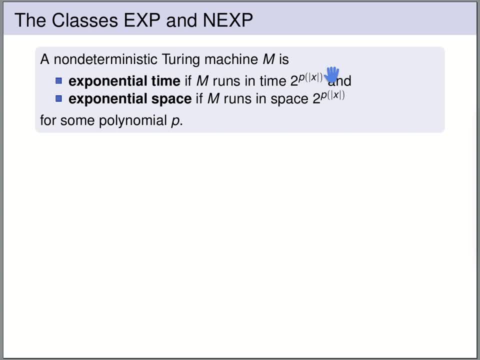 double and triple exponential functions, So we do not want that in the exponent. we have another exponential function. The base 2 is arbitrarily chosen. You can choose base 3,, 4,, 5, whatever you like, and it will not change the definition of exponential time. 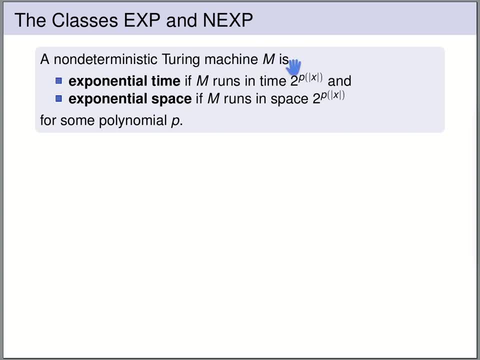 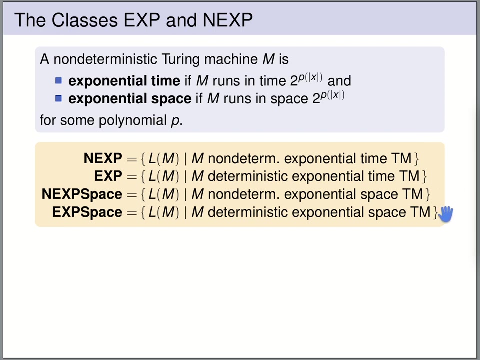 So, for instance, choosing base 4 is equivalent to choosing base 2, but multiplying the polynomial by 2. So changing the base does not change the definition of exponential time and exponential space. Now we can define exponential time and exponential space complexity classes analogously to the polynomial time and polynomial space complexity classes that we've already seen. 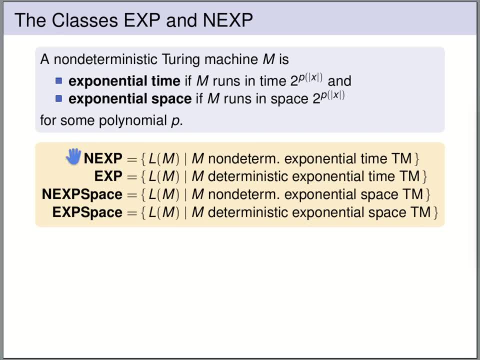 We have an exp consisting of all those languages accepted by non-deterministic exponential time Turing machines. We have a class exp consisting of the languages accepted by deterministic exponential time. The class nxspace consists of languages accepted by a Beast v pays the 我了解了 Adjusted place here. 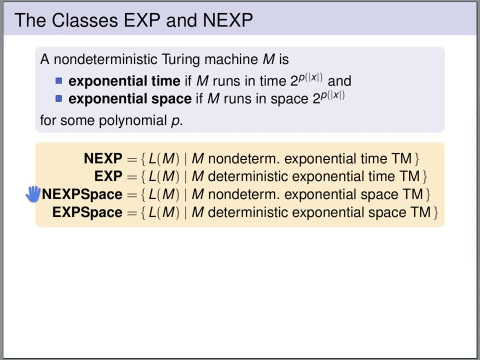 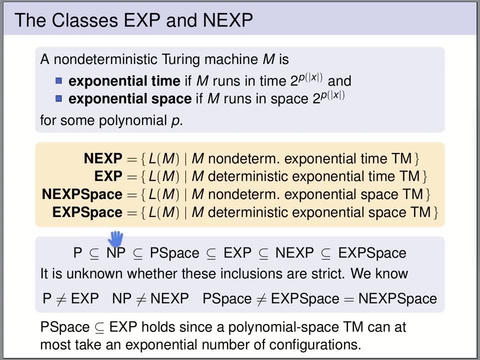 v the massa one ve of PSPACE. Now PSPACE must be a subset of EXP. so exponential time. If we have a Turing machine that operates in polynomial space so it visits only polynomial many places on the tape, there can only be exponentially many different. 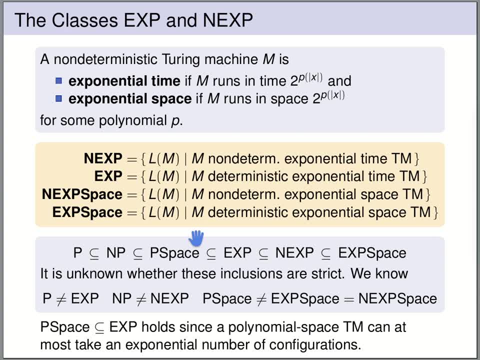 configurations for polynomial many places on the tape. Therefore, every polynomial space Turing machine must operate in exponential time. So PSPACE is a subset of EXP. EXP itself, of course, is a subset of N-EXP. so every deterministic machine is also a nondeterministic machine and N-EXP is a subset of. 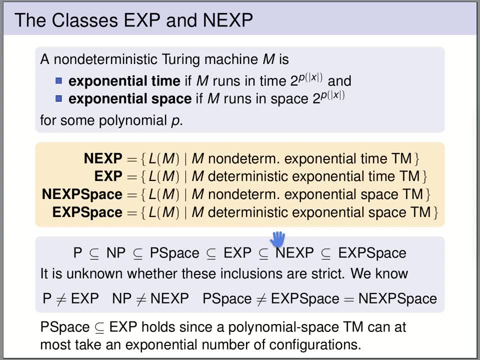 X-SPACE. If we have a Turing machine that operates in exponential time, so this can also be a nondeterministic machine- then Then it visits, in each time step, only one place on the tape, so it can visit, at most, exponentially many places on the tape. 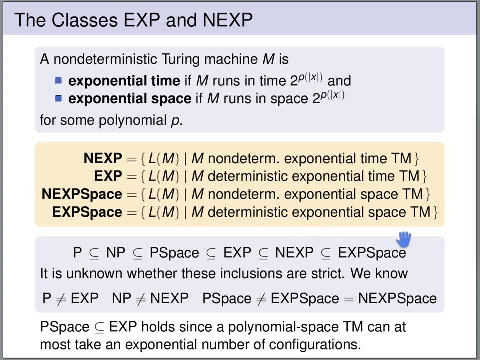 So any exponential time-turing machine must be exponential space, And what we use here also is we use Savage's theorem, namely that the x-space is the same as nx-space. If we have a nondeterministic machine that uses exponential space, then we can make a 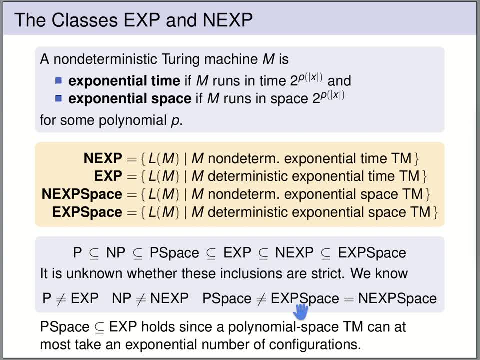 deterministic machine that uses exponential space. Recall that Savage's theorem said that whenever we have a nondeterministic machine that operates in space f, then we can make a deterministic machine that accepts the same language and operates in space f-squared. If you take an exponential function and you take the square, it's still an exponential. 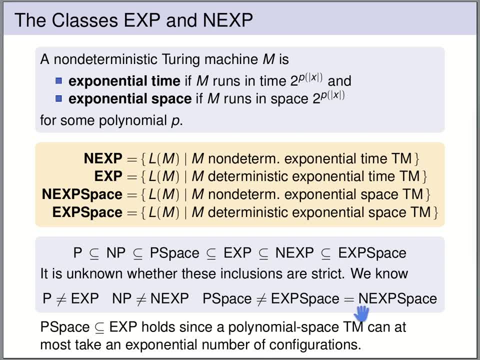 function. So x-space is the same as nx-space. For most of these inclusions it's not known whether they are strict, So actually we only know that p is a strict subset of exp. So deterministic polynomial time is strictly weaker than deterministic exponential time. 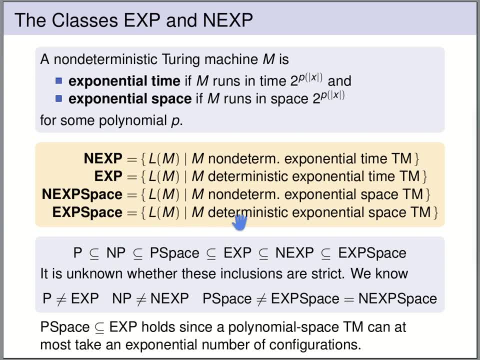 We also know that np is a strict subset of nexp. Nondeterministic polynomial time is strictly weaker than nondeterministic exponential time, And we know that p-space is a strict subset of x-space. So deterministic polynomial space is strictly weaker than exponential deterministic space. 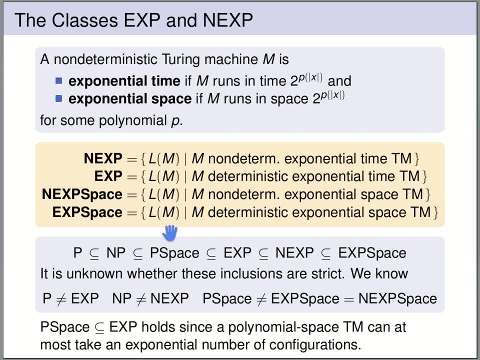 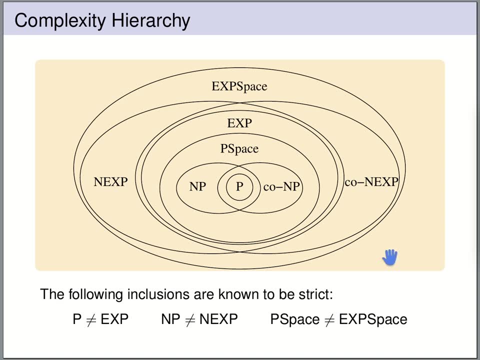 The other inclusions are not known whether they are strict. So for most of the inclusion it's open. It's open whether they are really strict inclusions. This picture summarizes what we've learned about complexity classes. We have in the middle our class P- deterministic polynomial time. np- nondeterministic polynomial. 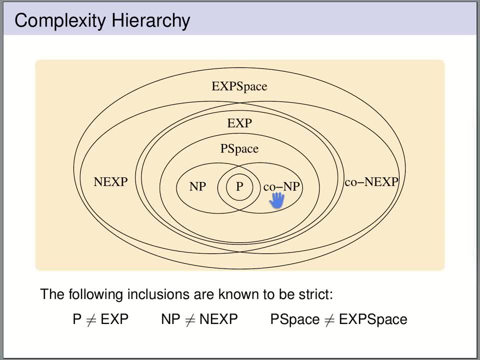 time We have co-np. A language is in here. if the complement is in np, Then the next larger class is p-space. p-space is, by the theorem of Savage, the same as np-space. So polynomial space, deterministic and nondeterministic is the same. 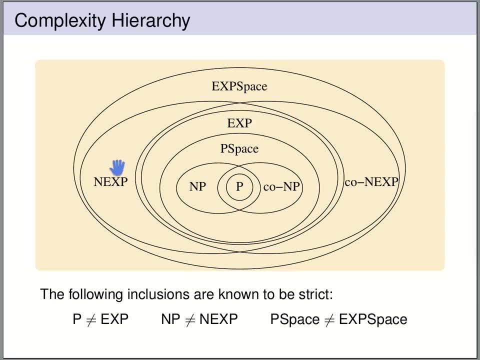 We have exp- exponential time, nexp, nondeterministic exponential time, co-nexp, So co-nexp is the class of languages for which the complement is in nexp. And we have exponential space, So co-nxp is the class of languages for which the complement is in nxp. 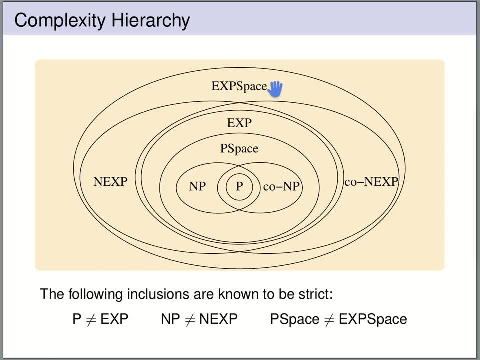 And again by the theorem of Savage, exponential space is the same as nondeterministic exponential space. Most of the inclusions in this picture are open whether they are strict. We know, as already said on the last slide, that p is a strict subset of exp. np is a.